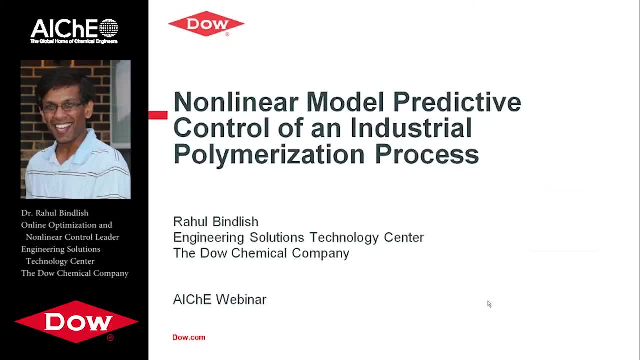 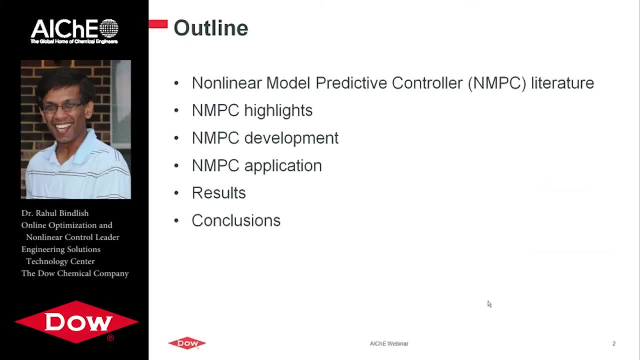 an industrial polymerization process And the way I want to present today as I'm presenting. I know John mentioned we don't have time for questions, So if you feel like you can even stop me. as far as I'm concerned, as long as the audio is going well. 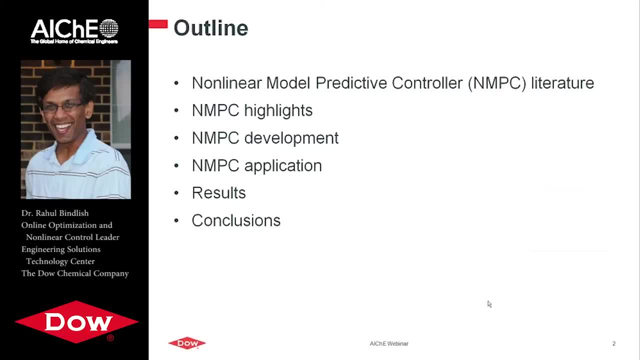 Here's a brief outline of what I'm going to be talking about today. I'll mention a little bit about the literature in this field, talk about the highlights for this problem and mention what we did for development and application, and then conclude. 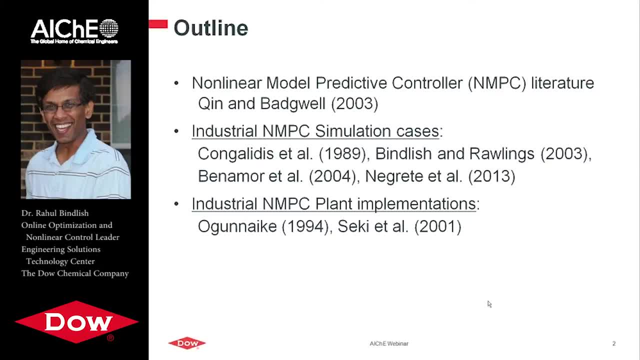 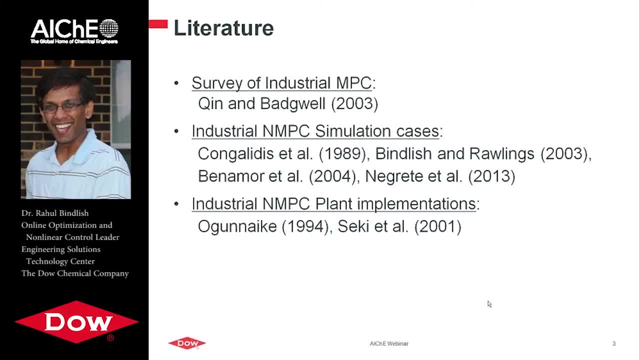 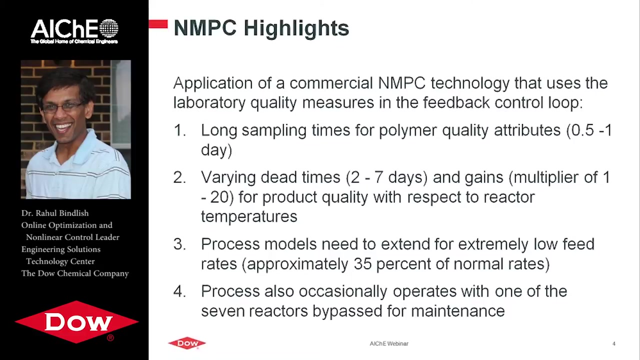 Some people have reported simulation cases and some advances in nonlinear model predictive control. for that There's a few papers that show results with actual planned data and implementations. All right, so this is a long slide that talks about the different highlights for this nonlinear model predictive control problem, but let me give you a little brief overview on how. 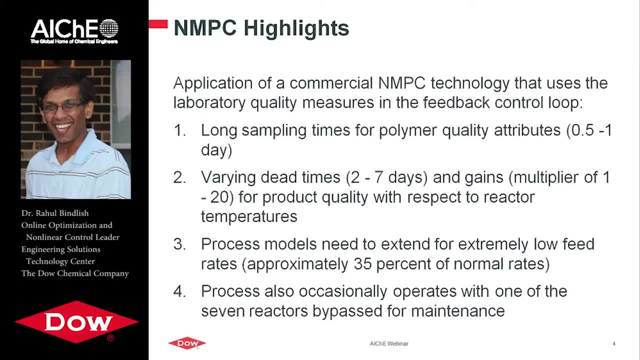 this came about. So at least at Dow, we have a long history of doing linear model predictive control And we have attained a lot of success with that. So we traditional tools to do linear model predictive control and those controllers have been running continually in closed loop and making a lot of money. 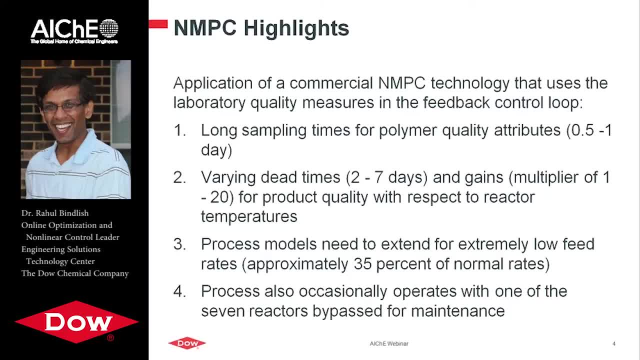 But we haven't had an implementation of a commercial nonlinear model predictive control technology in Dow, So this was chosen as a first pilot project to do So. we wanted to demonstrate that there was a need and a value case for a nonlinear model predictive control. 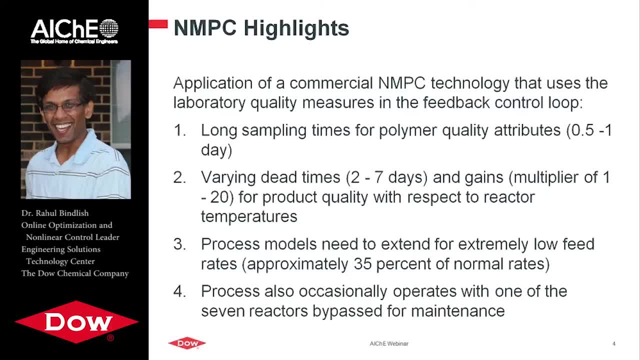 on nonlinear model predictive control compared to what we have been doing successfully for different plans and businesses. So as we picked a pilot project, we were also careful. I wanted to pick a pilot project where there was significant nonlinearity, So there was a case to use nonlinear model predictive control. 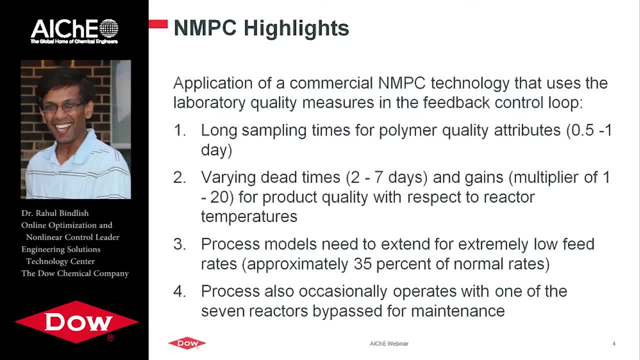 I didn't want to do a pilot project and then say, hey, here are the results, We are doing wonderful control and we are making lots of money. I wanted to clearly see the case for nonlinear model predictive control before implementing it. Basically, I wanted to answer the question. 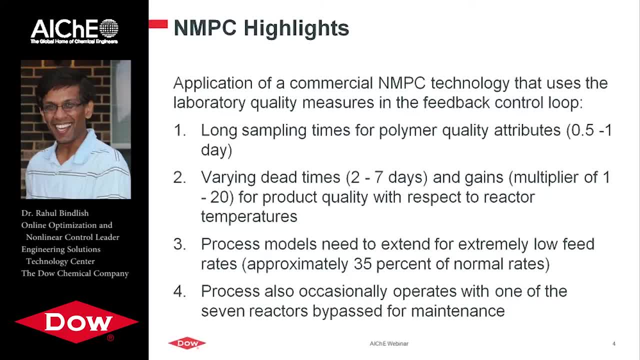 the problem does need a nonlinear model predictive controller, not a linear model predictive controller. So this talks about some of the highlights for the problem that essentially mention the nonlinearity in this process. In this case, we're doing nonlinear model predictive control for nonlinear model predictive control. 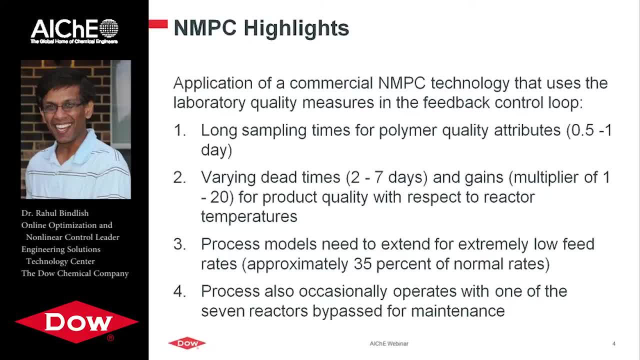 For a polymerization control problem And we are actually using the lab quality measures in the feedback control loop. So it's not an advisor whereby we come up with a reactor temperature profile and then we maintain that temperature profile in the controller. So it's not doing that. 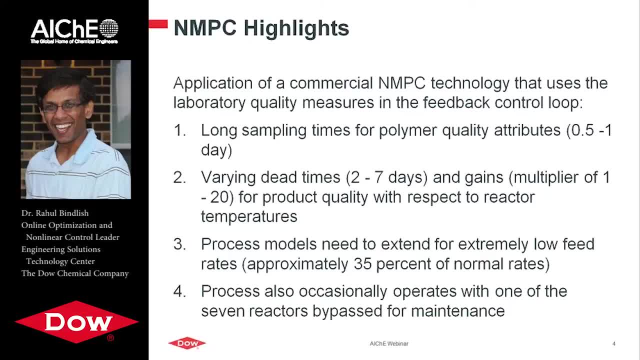 And within that control problem it has significant nonlinearities and challenges and interesting aspects. So there are long sampling steps, Some of these times for the polymer quality attributes. some of them are sampled only once a day, The others are sampled twice a day. 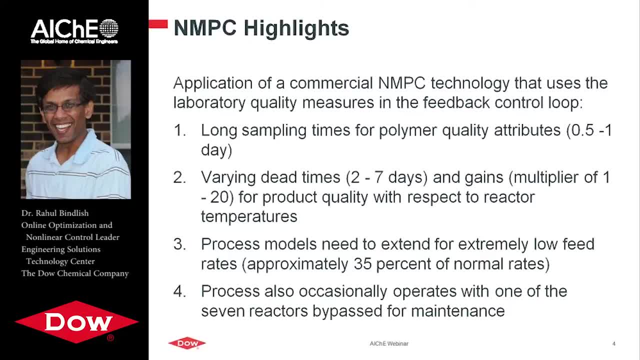 We got varying dead times. depending on the process conditions and rates, The dead times could vary anywhere from two to seven days. The gains are varying a lot, from one to 20, depending on reactor temperatures and feed rates And then the process models. 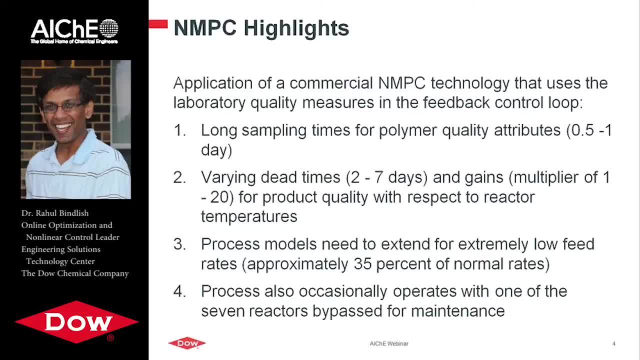 need to extend for extremely low feed rates. When we first started building this controller, we were told they would run typically about 70% of the nominal rates And lower than that. they wouldn't want this controller to run, And as so, it's been a learning and a journey in progress as we have gone. 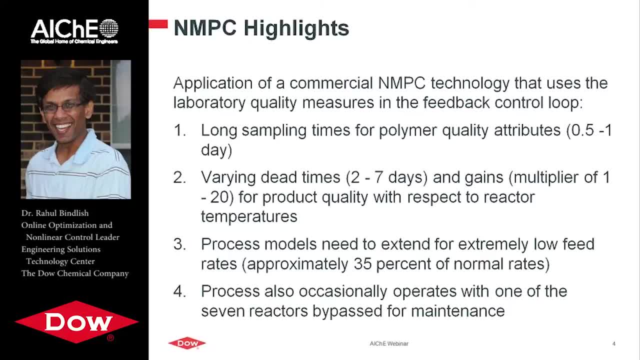 through some of these objectives over the last two years. This controller was first implemented in October 2012.. And since then we have learned a lot. So what we learned? after the controller ran for like eight or nine months, we learned there was a need to run this controller at lower feed rates. 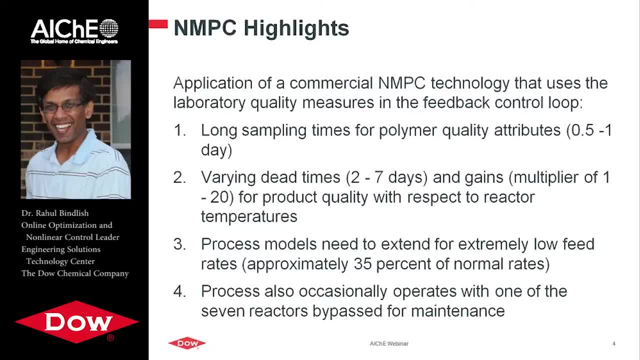 which was approximately 35% of normal rates. because of the business condition And because of the initial success of the controller, they would rather have this controller run at those really low rates instead of having to go back to the previous way of running things. 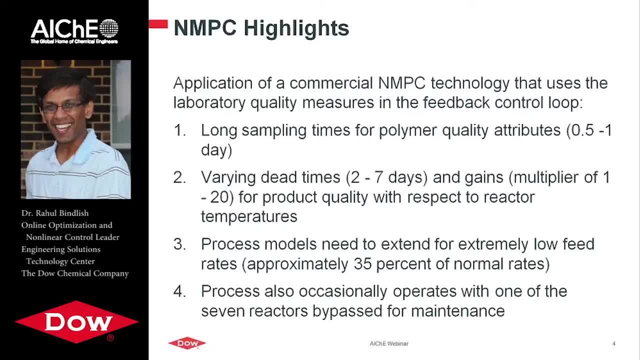 When we, when we first commissioned the controller, the initial controller was built for the seven reactors in series, And what we were told back then is sometimes the reactor is taken out of service for maintenance and that's a short period of time, So there's no need to run the controller in that period of time. 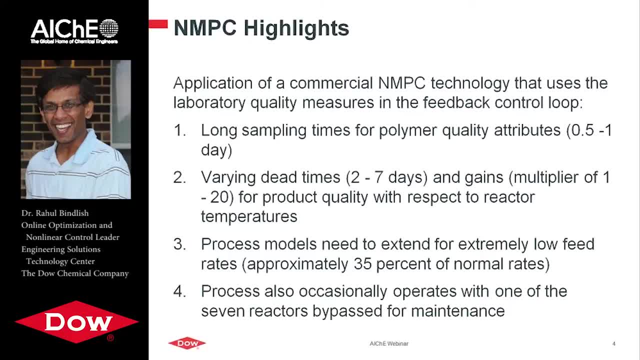 But since then, when the business conditions were not very well were not good. we also had a need to run the controller for a long period of time, when they ran the process with only six reactors instead of seven. So, in short, especially the last two bullet items. 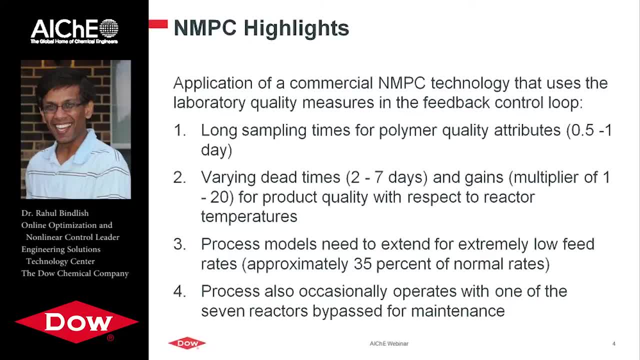 they signify some of the things that happen in real life In an industrial case. we build a controller, we do things and then you know, in my career here, and what I've realized is whenever we implement anything, things always change, because we cannot predict the future. 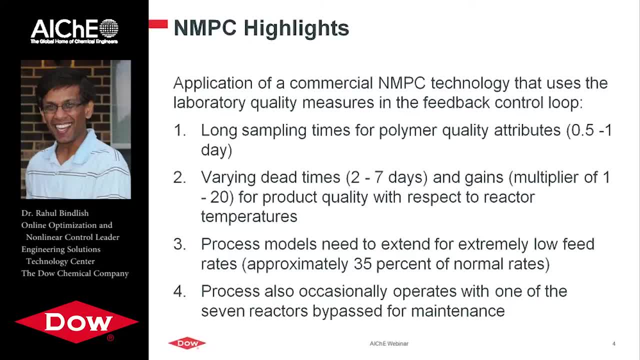 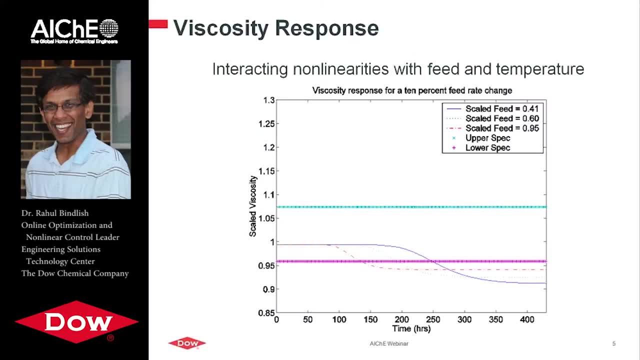 Okay, Thank you. But the nice thing with this technology is it allows us to still realize value. So I talked about significant nonlinearities. So when I'm talking about significant nonlinearities, there are significant nonlinearities and dead time gains, settling time. 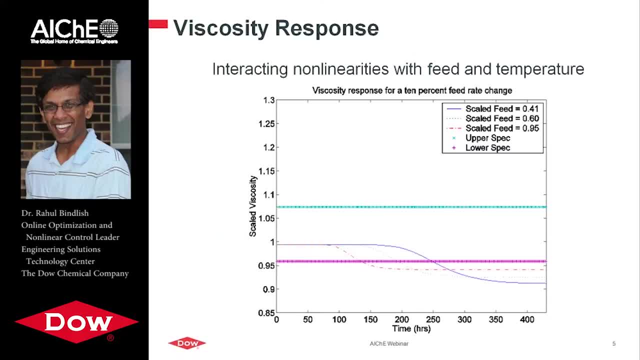 So it cannot be controlled using a linear MPC. We verified that. We did a technology assessment And realized that this problem needed a nonlinear controller. But this graphic just shows the extent of nonlinearities a little bit. So on the Y axis you've got scale viscosity. 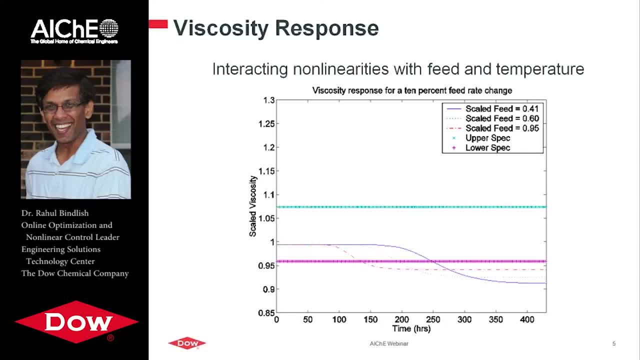 which is a polymer quality attribute or scale, So you don't get to see the real numbers. Then the horizontal line are the spec limits. So what I'm showing here, the blue line is the variation in viscosity if the feed rate was to increase 10% from where it is. 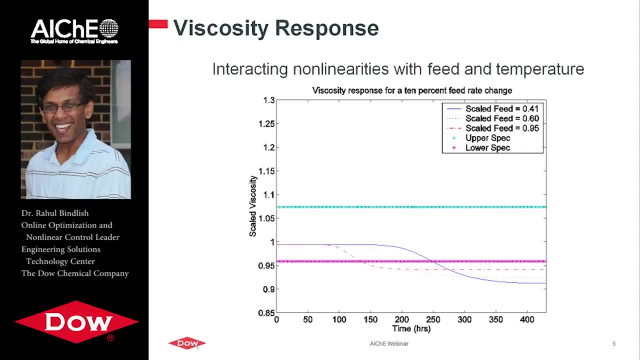 So it has a dead time of about 200 hours or so and then it dips down And it would cost if you didn't do anything. it would basically go below the lower spec limit. So it shows how the dead time is changing depending on the feed rates. 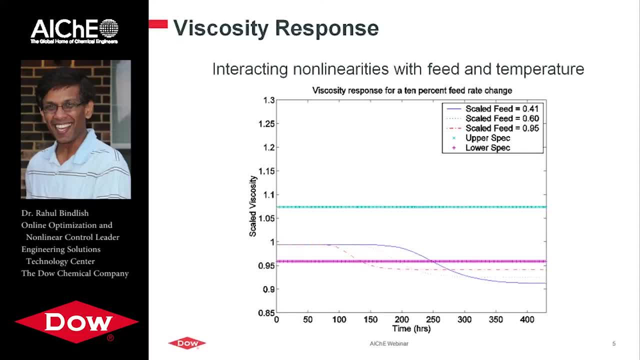 or a 10% feed rate change And the gains are changing too. It's just a simple graphic that kind of tries to highlight the problem. So the one thing to notice here is the dead time and the settling time right, So the dead time is like 200 hours. 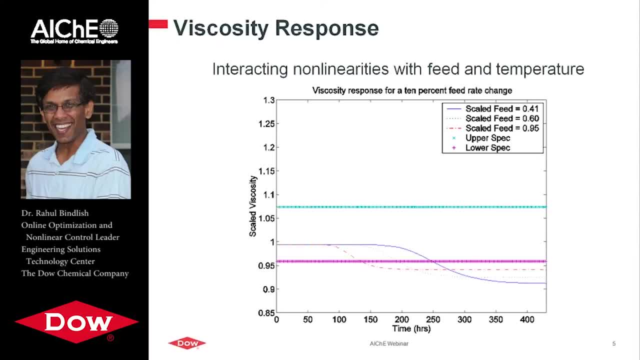 It could be 100 hours, So you don't see anything happening in the process. So the models have to be accurate. They need to capture what is happening, They need to capture the nonlinearities, Otherwise you're going to have significant spec issues. 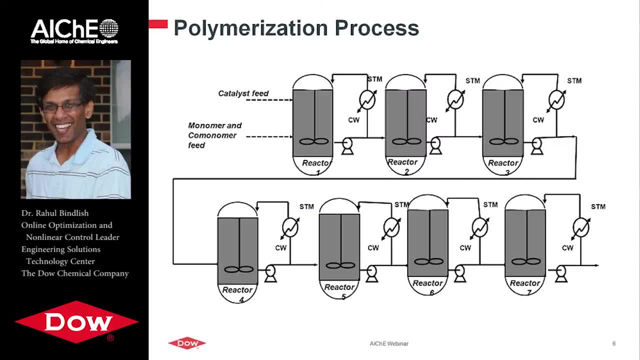 So graphic on the process itself: Seven reactors in series. Each of the reactors can be heated up or cooled down by using steam or cooling water. We've got catalysts coming in. We've got monomer and co-monomer being fed in. 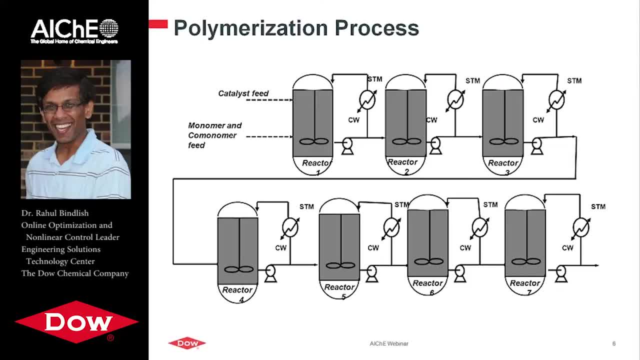 And that's what's going on, And we've got the product coming out of the seventh one, All right, So we're going to move on to the next slide. We're going to move on to the next slide. We're going to move on to the next slide. 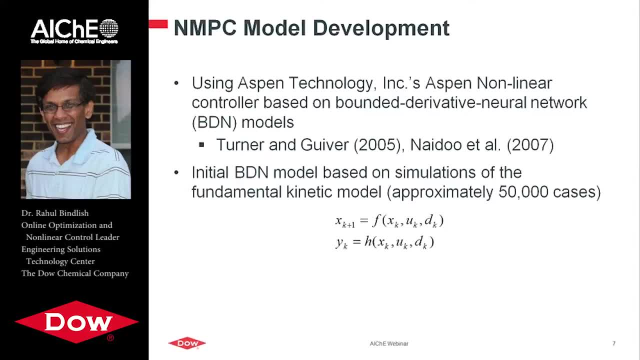 All right. So when we are in grad school- I mean, a lot of you are in academia, Myself was in grad school at University of Wisconsin and I did my thesis in this area- Then you have all the flexibility. You can basically build your controller or write your equations and do it in whatever format. 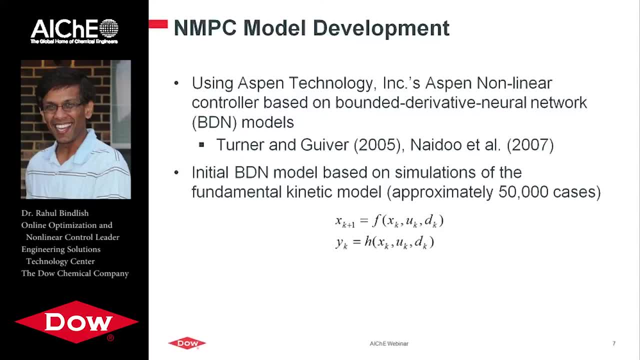 You can write Fortran code, MATLAB code and such and make a theoretical advance, But there are different challenges. in an industrial setting We have to use a commercially sustainable solution, So it should have the appropriate interface and the solution should be able to migrate. 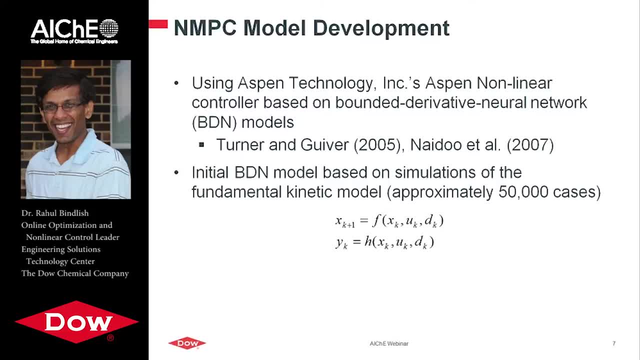 to new operating systems and such. So in this case we are using Aspen-Tex nonlinear controller based on the boundary derivative neural network models, And there's a couple of papers in the literature: Turner and Guyver and Naidoo et al. 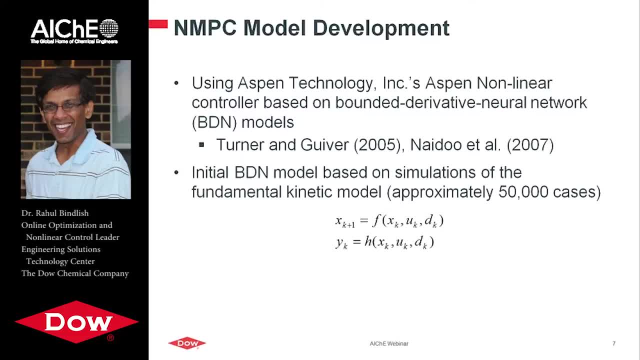 that outline the model, All right, So I'm going to go ahead and show you a little bit of the mathematics behind it. So for this process we did have a kinetic model. We had a kinetic model in Fortran that had been used by the business for a long period of time. 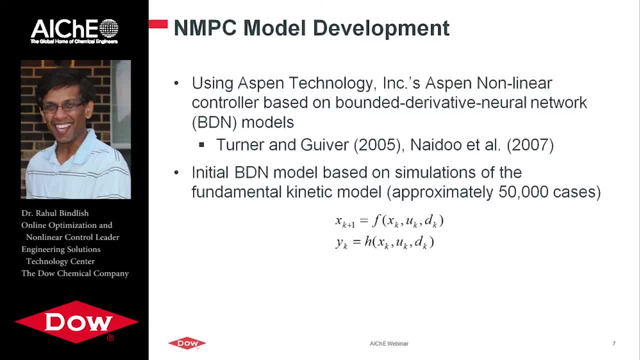 because they are using that kinetic model for process development and validation. So what we did is we used the kinetic model and we did lots of simulation cases to construct our BDN models. In this case, we ended up choosing 50,000 cases to cover the operating region of interest. 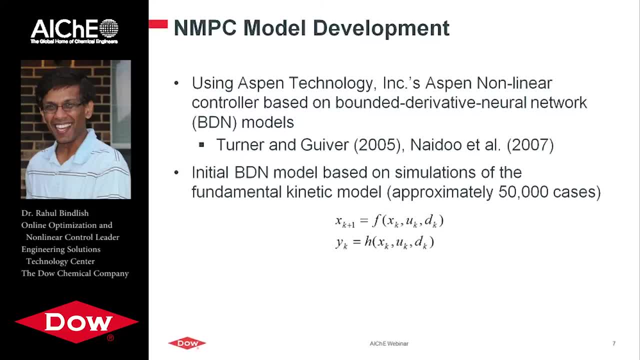 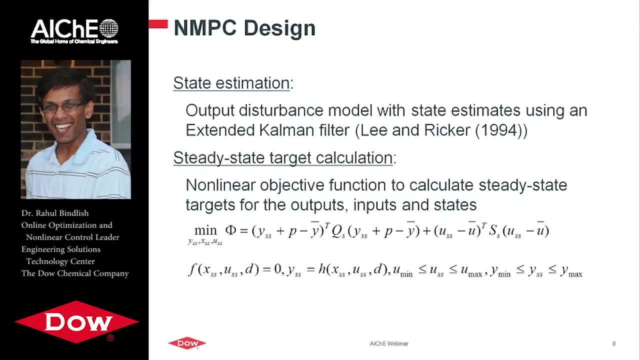 And essentially we have a state space kind of formulation where x's are the states and u's are the manipulated variables. These are the measured disturbances and y is the output that we're trying to control. Like in any model predictive controller, there's three aspects here. I want to mention how it is done. 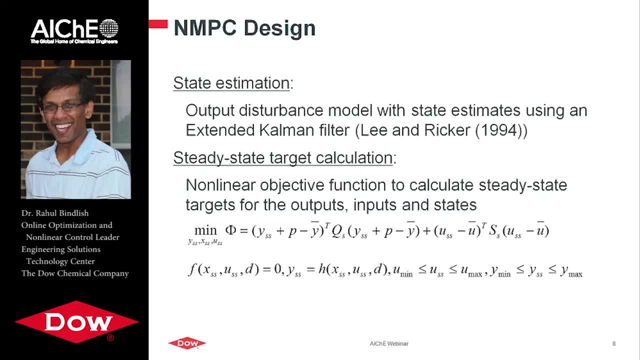 in this nonlinear model predictive controller. The first is state estimation. We're using an output disturbance model with state estimates, using an extended common filter with covariance updates. That's what we're doing And there's a paper that mentions that. Lee and Ricker 94 paper talks about that in detail. 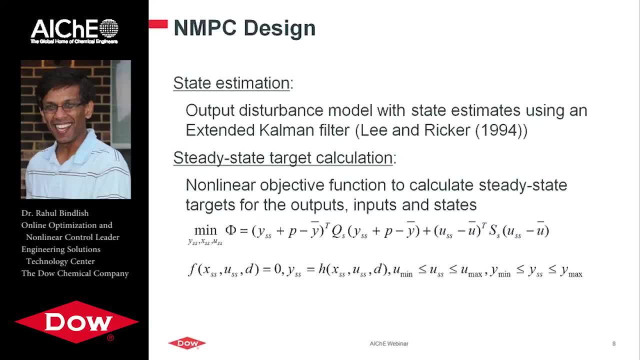 For the steady state target. we're going to use a nonlinear model predictive controller. We're going to use a nonlinear model predictive controller For the steady state target calculation. we have a nonlinear objective function to calculate the steady state targets for the output inputs in the states. 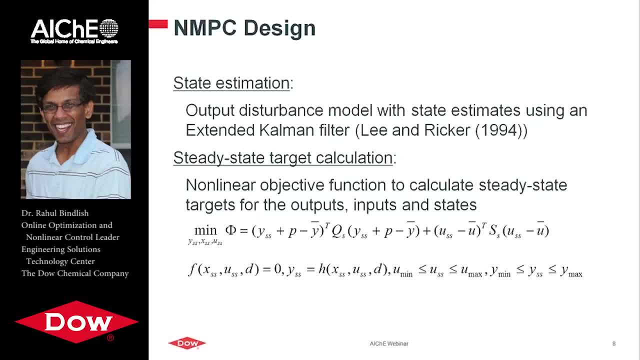 And in this objective function essentially we are minimizing the deviation of the steady state prediction from the desired value and balancing that against how much we would be moving the output inputs or the manipulated variables from their current value. That's the desired values. We really don't want to move the reactor temperatures unnecessarily. 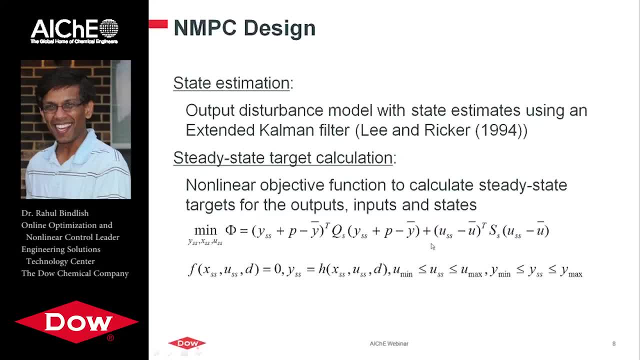 So that's the tuning we do. In addition to that, we have the model equations. We're making sure they get satisfied for the states as they propagate. At steady state it'll be zero, The derivative will be zero. And we also make sure we have the model equations for the output variables, the measurements. 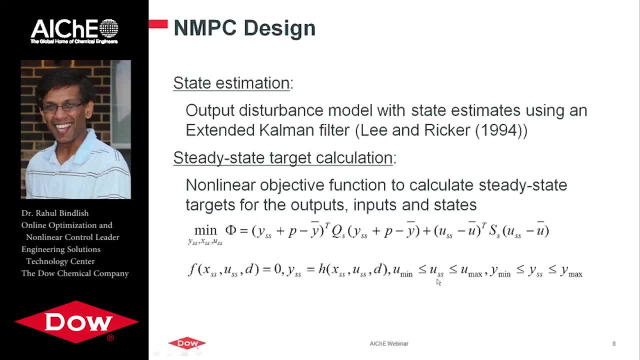 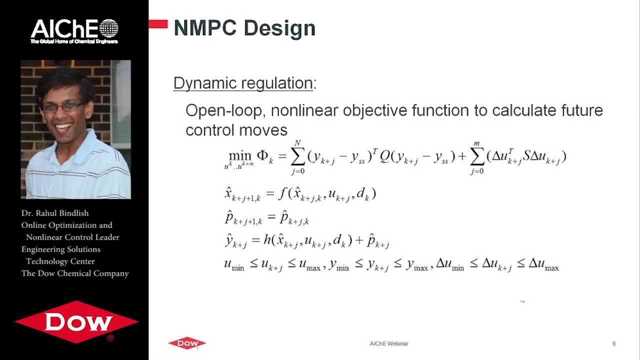 While we satisfy the constraints on the inputs or the manipulated variables, and the outputs too. The third part of an MPC controller would be the dynamic regulation, And in this case also we're solving an open loop nonlinear objective function to calculate the move plan. 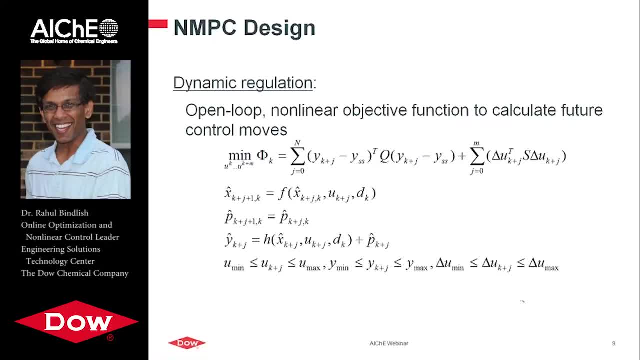 And in this case also, we're solving an open loop nonlinear objective function to calculate the move plan. And in this case also, we're solving an open loop nonlinear objective function to calculate the move plan And we're basically minimizing the deviation of the output measurements. 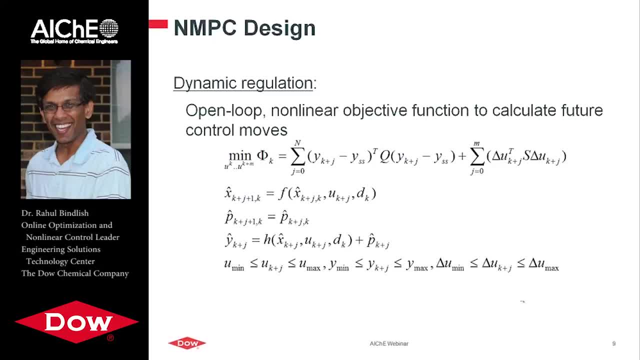 from the steady state target over a period of time over the horizon, And we're also analyzing the rate of change of movement, of how much we're moving the inputs from the current values. And while we do that, we are satisfying the model equations, the states of the model. 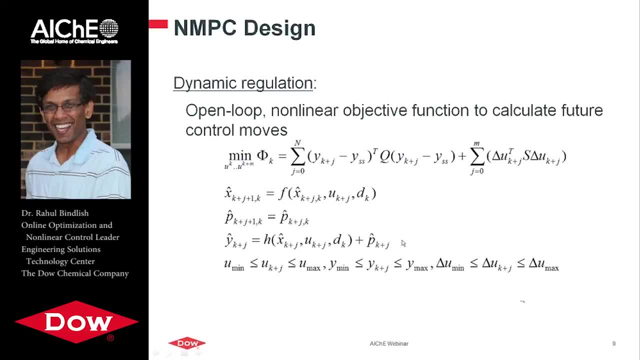 the output disturbance states and also the output measurements. We're propagating those. We're propagating those equations and making sure they get satisfied. And we have the constraints on the inputs or the manipulated variables, outputs and the rate of change of inputs too. 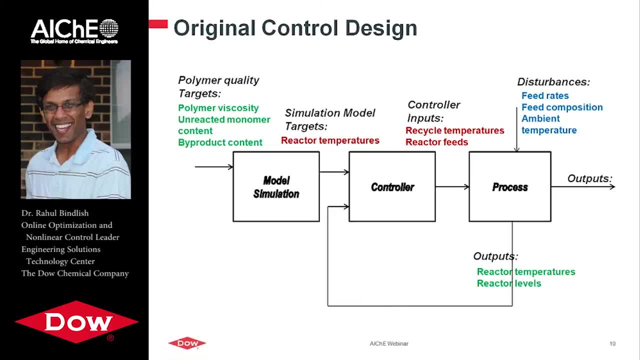 Okay, So a natural question that should arise in anybody's mind would be: if the process is so nonlinear, before you implemented nonlinear MPC, what was going on at the plant? There was no linear controller, so what was going on right- So in some ways some would even classify it as a nonlinear controller- was already running. 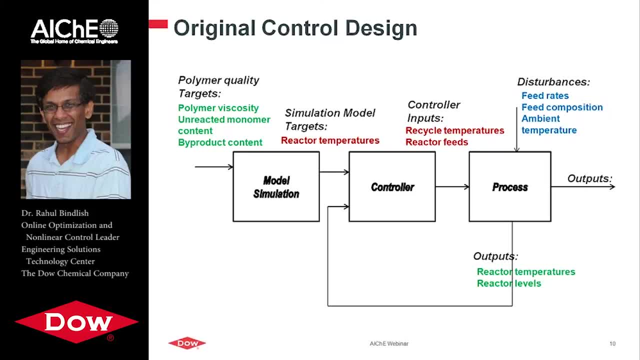 So let me talk about what was going on at the plant, So what we had at the plant back then. we had the model and it was being run in a simulation mode and it was providing the reactor temperature profile. So that model was running. 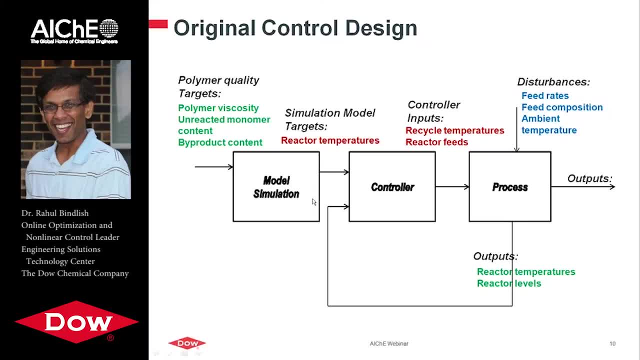 And it would. It would come up with a reactor temperature profile that needs to be implemented at the plant, So that reactor temperature profile then would be implemented in the plant using the DCS controller that allows us to do that. So we are basically maintaining the reactor temperatures. 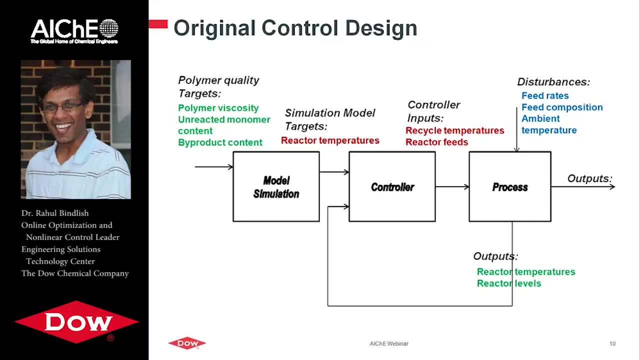 and the reactor levels by manipulating the recycled temperatures and reactor feeds. So that was in the feedback control loop: manipulating the temperatures and feeds, the recycled temperatures and reactor feeds, to maintain the reactor temperatures And we were keeping the levels sort of constant. So that's what was going on. 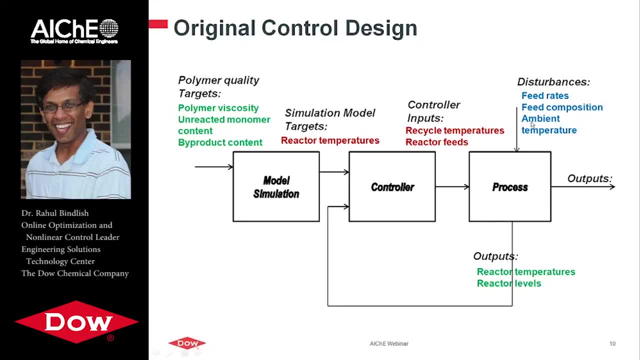 The process was getting disturbances with feed rates and composition and ambient temperature And every time a lab measure came in for polymer viscosity on unreacted monomer content, then basically an adjustment was made to the temperature profile And we were able to get the temperature profile manually if needed. 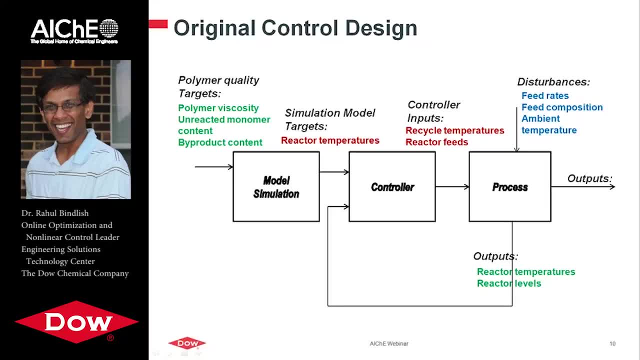 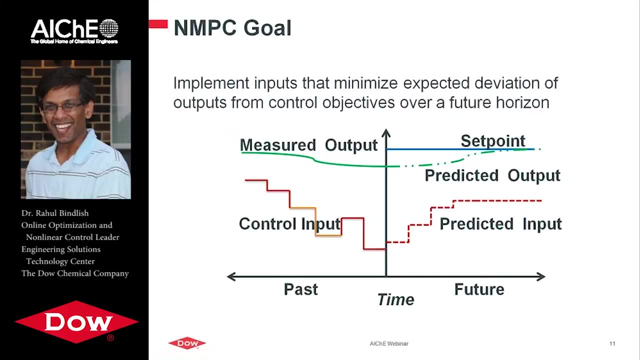 But there was no direct feedback control loop, It was just open loop simulation that was sending that guidance to the controller. A little graphic on what's going on in an MPC scheme of things. We are essentially trying to minimize the expected deviation of the output. 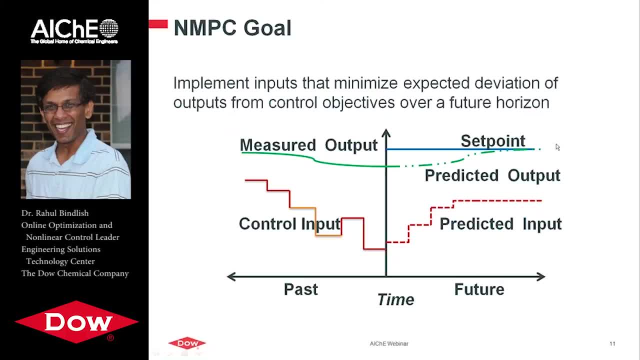 from the control objectives over a few days. So that's what we're trying to do with the MPC scheme And we're trying to minimize the future horizon, And in this case the horizon is longer than the settling time. So we are making sure we are covering the entire span. 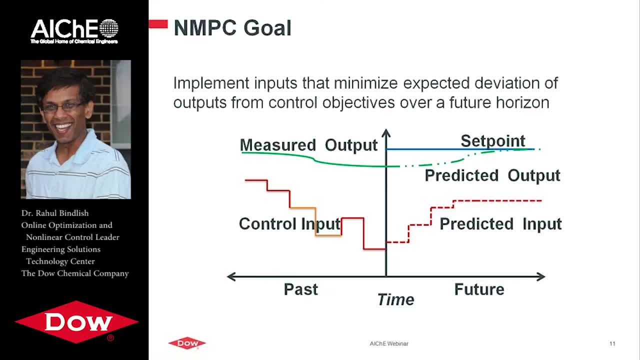 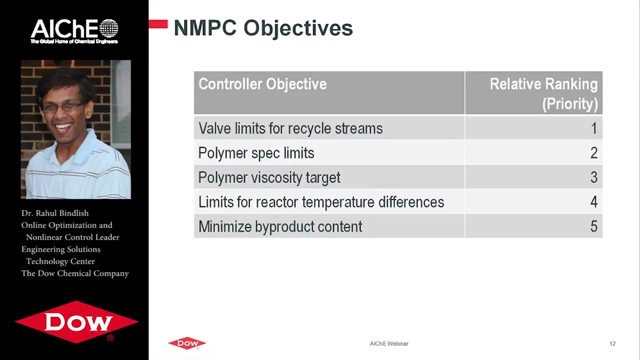 And we are minimizing how much we're moving the control inputs or the manipulated variables. And every time we are calculating this move we implement the first move And then in the next controller execution time we recalculate the move plan. So let's talk a little bit about the controller objectives here. 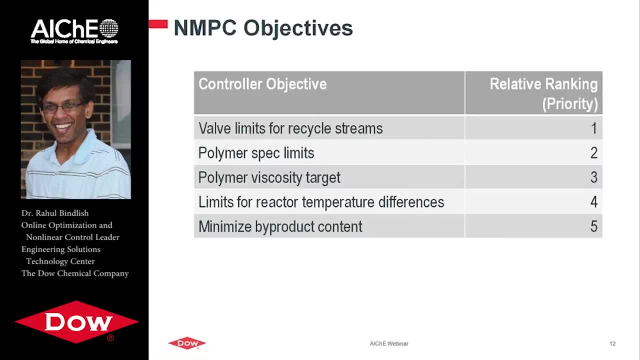 So this table shows the relative ranking or priority for the different controller objectives. So things like physical limits, the valve limits for recycled streams, we need to make sure they're honored so we don't try to do something that's not physically attainable. 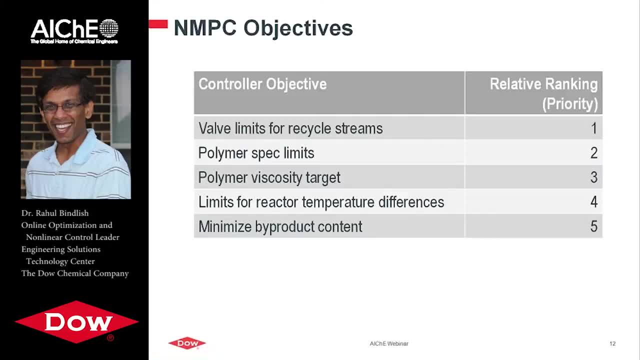 That's going to have the highest priority. The polymer Spec limits: They're very important. The polymer viscosity target in this case is the next important limit. Then we also have limits for reactor temperature differences. What those limits are doing is essentially, we don't want to heat up in the first reactor. 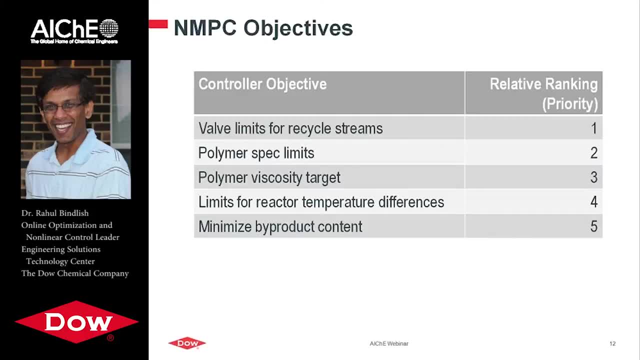 and then cool in the second reactor and then heat up again in the third reactor. We want to avoid having that kind of zigzag profile if we can, So we have something called reactor temperature difference CVs that allow us to achieve that. We added a. we ended up adding another controller objective recently. 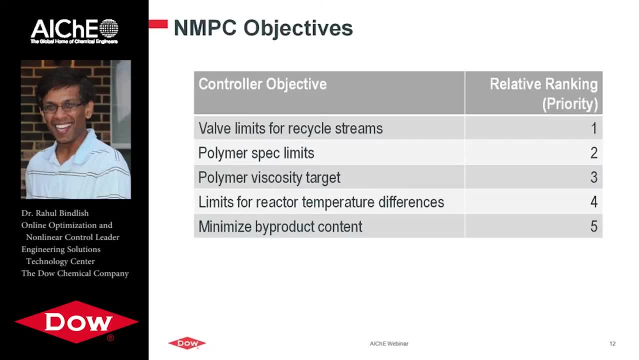 It's been about a year or so, And that's to minimize the byproduct content, And this was something we didn't have in the initial controller design. We didn't even have a lab measure for it, But, based on the success of this controller, we ended up adding a lab measure for it. 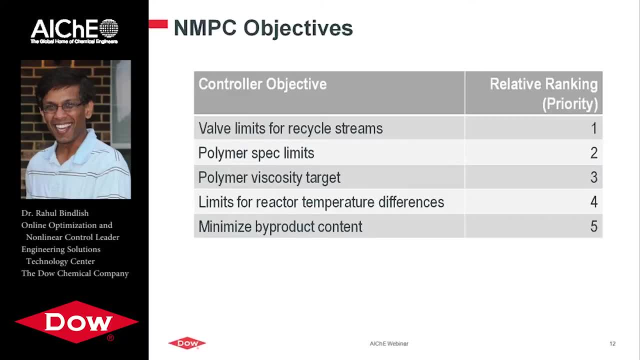 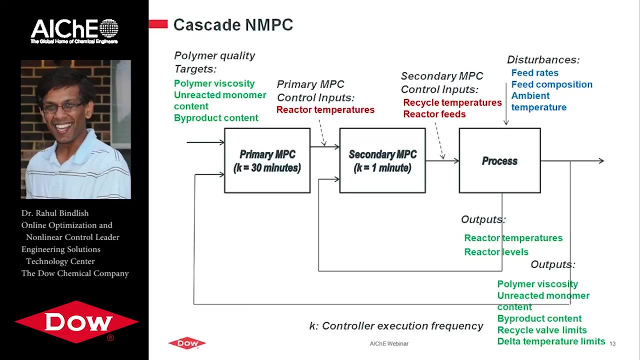 and also added it as a control. It gives us better economics when we are able to minimize byproduct content. So the nonlinear control design- in this case we have a cascade nonlinear control design. So the very first question that would arise in a lot of you all's mind would be: 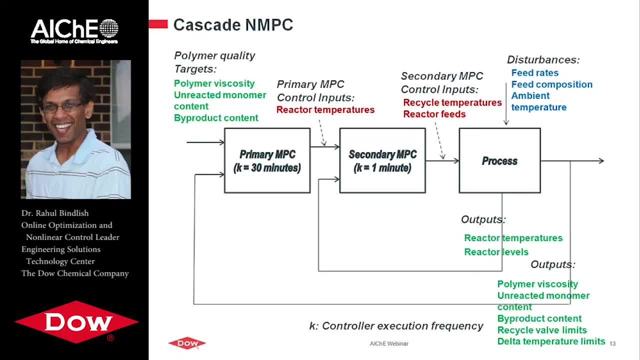 why a cascade, nonlinear control? Why not put it all together? A couple of reasons. One of the main reasons is the computational need reason. If you put everything together in one controller, it's going to be very hard to realize it computationally in real time to achieve the objectives that we want to achieve. 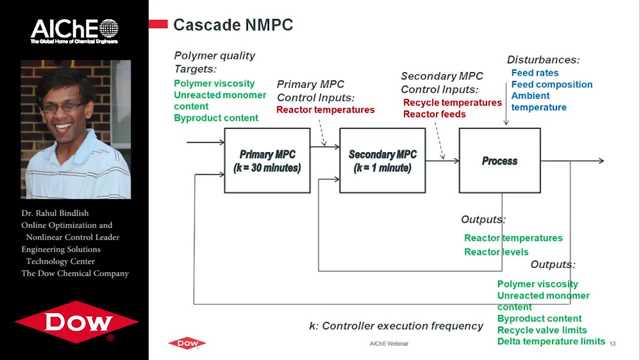 So we needed to break it for that reason. So let me talk a little bit about that, okay, And also the linearities and nonlinearities where they belong. So I'll mention all that. So let me talk a little bit about that. 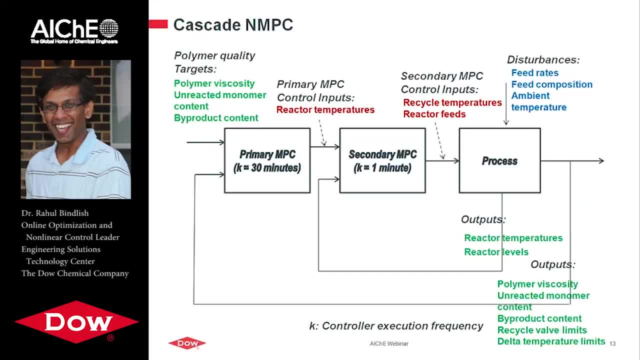 So the reactor temperatures themselves. with the disturbances coming to the plant. they have a settling time with respect to recycled temperatures and reactor feed that may be anywhere from three to six hours depending on rates and process conditions. We need faster disturbance rejection and the ability to maintain reactor temperatures. 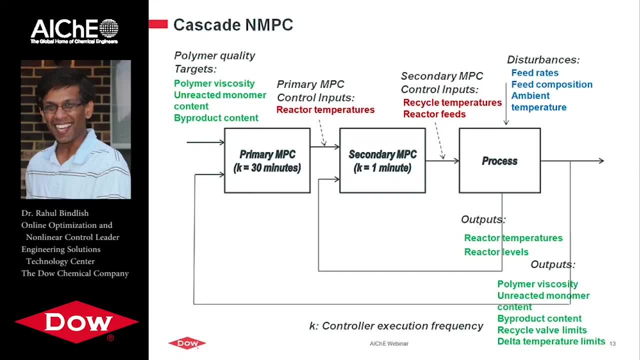 So that controller is running every minute. The models for that controller are the secondary MPC or more or less, are close to linear, and that's the reason in the past we were able to achieve those objectives even using a DCS, even in the DCS. 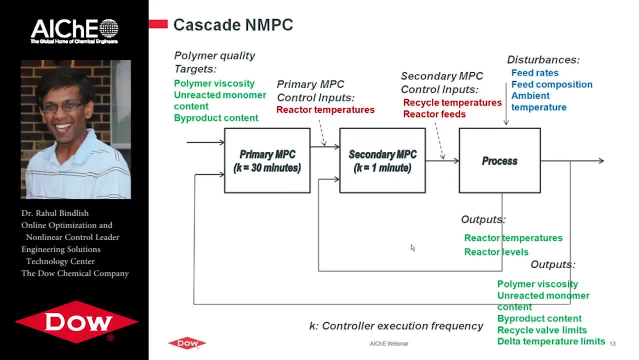 even without using a linear model predictive control. But with a linear model predictive control we are doing better than what we were doing with the DCS-based scheme Now on the secondary loop or the primary loop, whereby in the past we just had a simulation model. 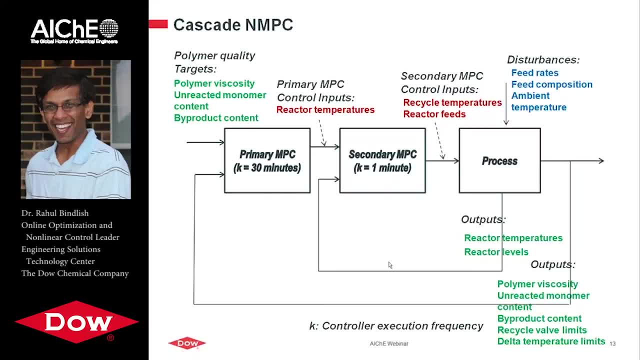 that was running and coming up with a reactor temperature profile. those models are the ones that are significantly nonlinear. So that's the primary MPC. The goal of that primary control MPC controller, which is extremely nonlinear, is to control the polymer quality attribute in a closed loop. 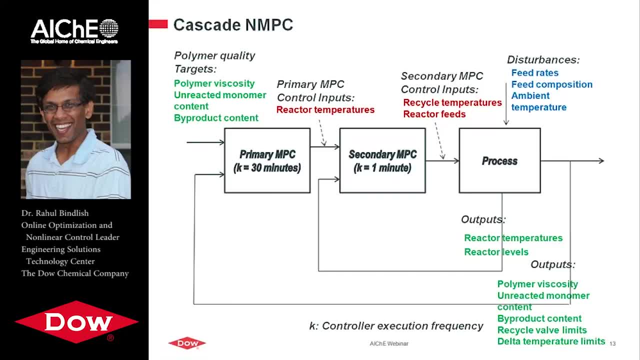 So the attributes that we are looking at are polymer viscosity, unreactor, monument content and byproduct content. These quality attributes have a settling time of anywhere from 10 to 15 days, so, depending on rates and conditions- And we are measuring them only- either once a day or twice a day- 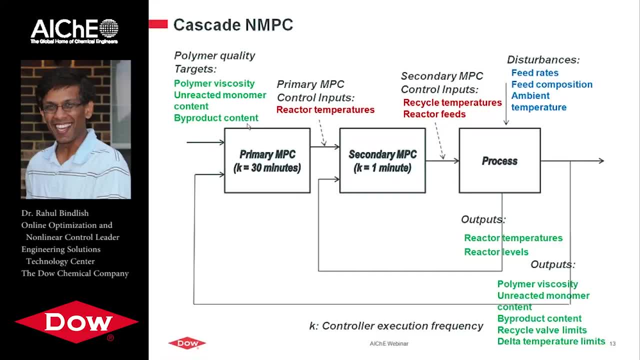 So, given that we are going to be able to do that, We don't really need as fast a disturbance rejection and we are able to get by running by running that controller only once every 30 minutes, As mentioned before. initially, the byproduct content was not. 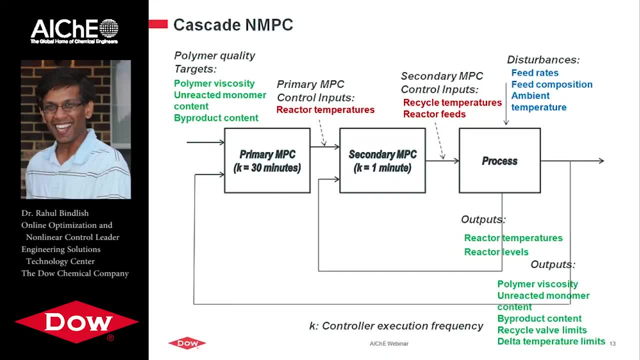 in the original scope of the controller. We ended up adding it after we had initial success with the controller and we got a lab measure for it. Both controllers are due model effects of the measured disturbances that enter the plant, which may be in the form of feed rate disturbances, composition disturbances. 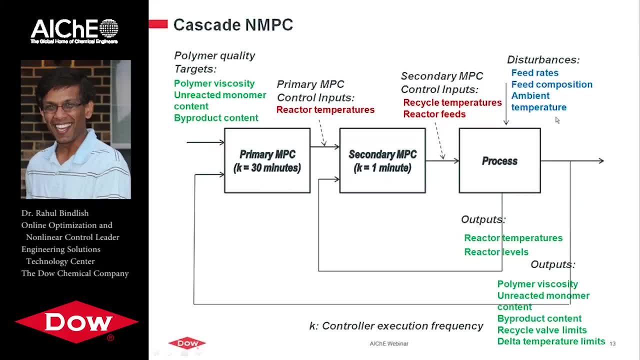 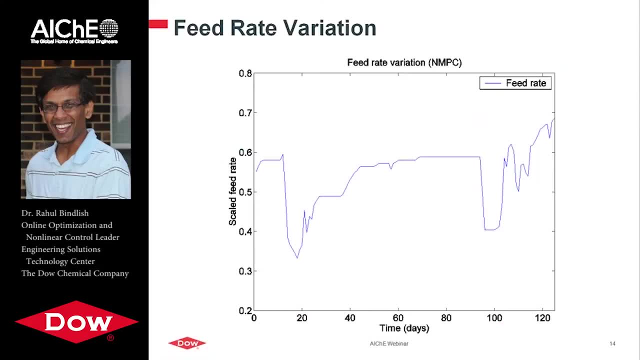 and ambient temperature. All right. This graphic, or this, gives an idea of how much. so what's the problem here? right? If nonlinearity is nonlinearity, but if the process doesn't change, then the nonlinearity is not as big a problem, right? 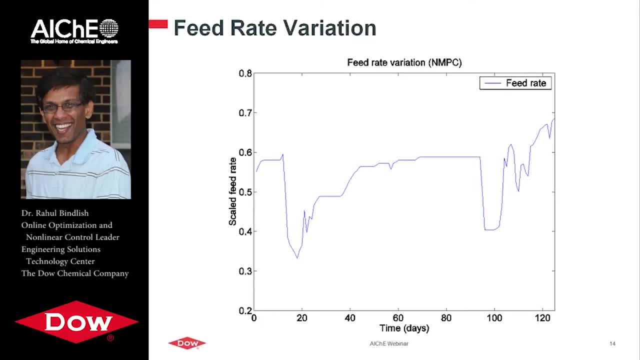 So the reason. so if you look at this graphic, what I'm showing here is this is the normalized feed rate through this process. It's about 60% here and then it suddenly drops to about 30% then we, then they end up raising the rates back up to 60%. 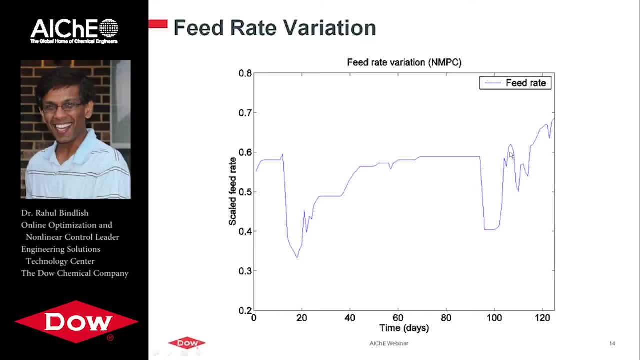 And if they stay there, then it suddenly drops again and they raise it back again and they end up being raised again. So what's happening here? is this the place where this plant is situated in our site. it gets impacted by upstream plants and also gets impacted by downstream plants. 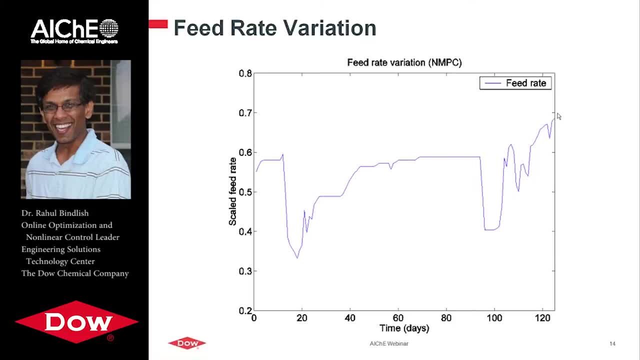 So it's in the middle sort of So because of that, and so it gets impacted by disturbances everywhere, so it has to undergo a lot of rate changes. So in this case we have a lot of rate changes. In this case those rate changes are significant and severe. 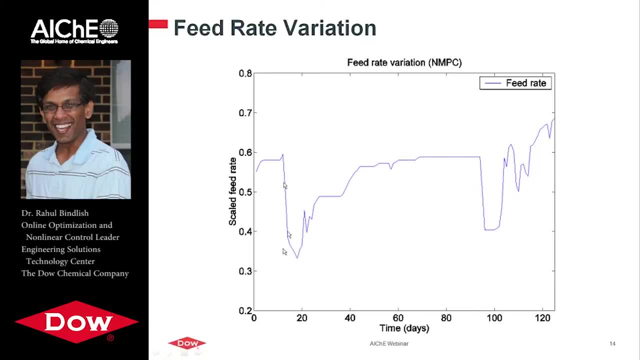 especially if there's a plant trip and such. In this case, this is a significant speed rate disturbance and that is going to impact the polymer quality coming out of this process. So if you look at the X axis, then you're going to be saying: okay. this is about four months of data. So you're going to be saying, okay, this is about four months of data. So if you look at the X axis, then you're going to be saying, okay, this is about four months of data. 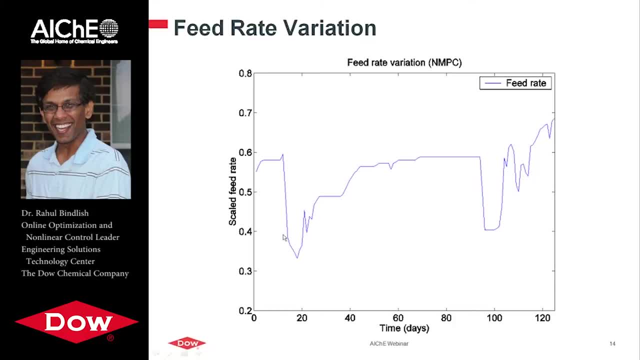 But you've got to realize these disturbances are happening over 20 days or so, but the settling time of this process for the polymer quality attributes can be anywhere from 10 to 14 days. so these are like sort of fast-moving disturbances for that settling time. 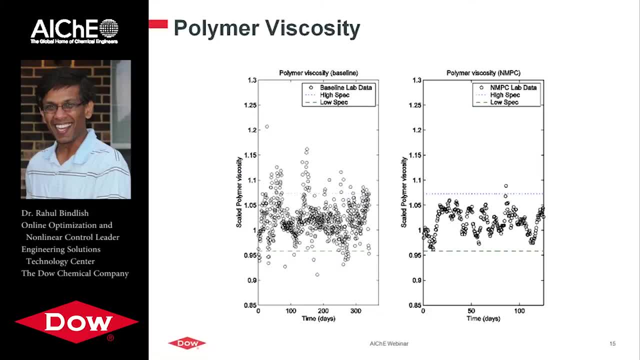 So the initial project, when it was chartered it was, the goal was to show better improvement in control, especially for polymer viscosity. That's how the project was chartered. So this shows baseline data, selected annual data from last year. 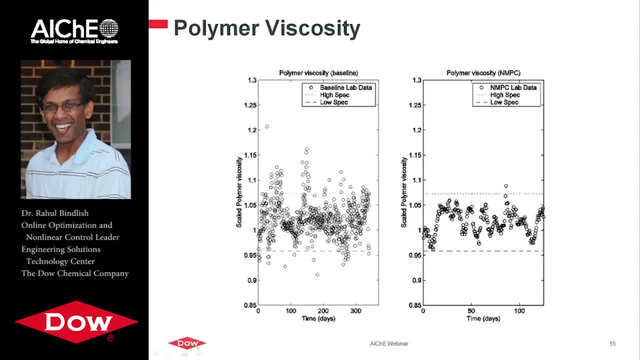 the year prior to doing this project. This shows how the viscosity was doing. This is upper spec limit. This is the lower spec limit. It shows how it was wandering off from the spec limit and also had a wider spread After the controller has been implemented we have had in this case. 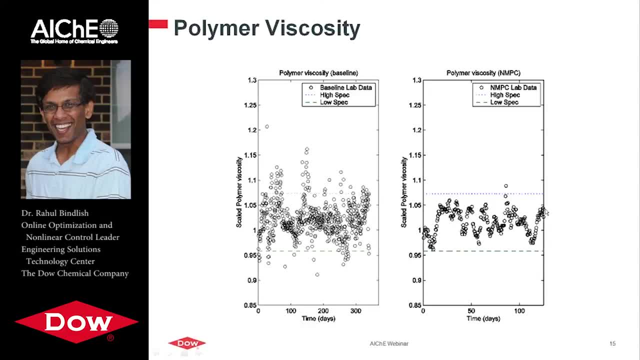 this is like four months of data, but we have even collected more data in the last two, three years. There have been much lesser excursions, maybe only a very few handful, and we also have a much lesser standard deviation, if you may say, for polymer viscosity. 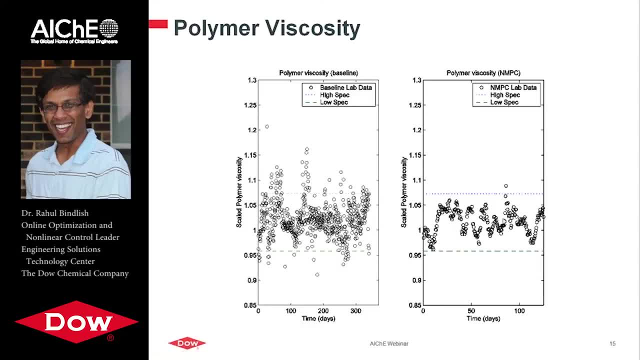 So we have tighter control and lesser excursions from the spec limit. So that baseline was collected for the case when the nonlinear model was running continually and was suggesting the profile to the plan, and the profile was the only thing, the reactor temperature profile was the only thing that was in closed loop. 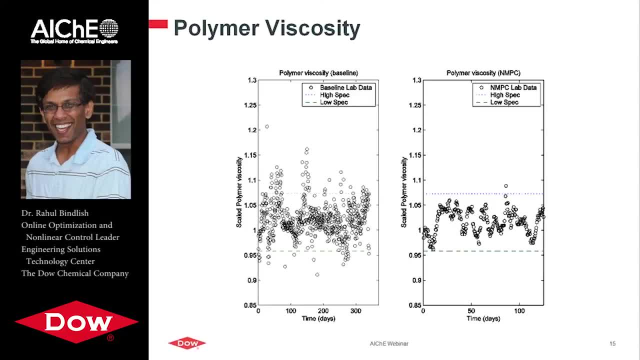 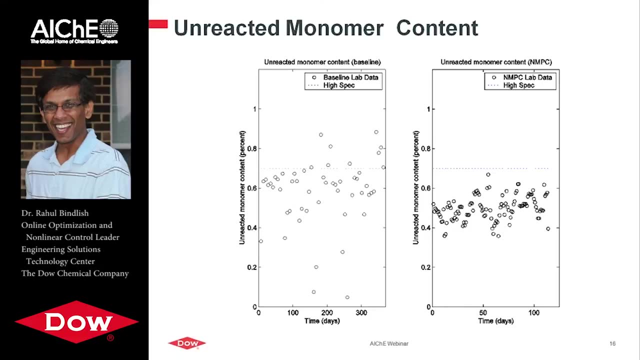 not the quality attributes, but the nonlinear model itself was running continually and that profile was fine-tuned manually. So the second objective, or the important polymer quality attribute, is the unreacted monomer content. The unreacted monomer content. the graph on the left side shows the baseline data. 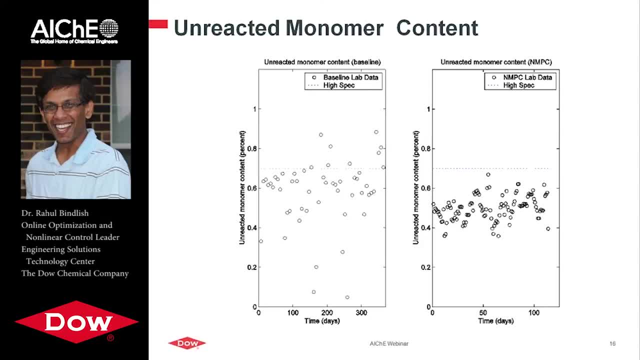 In this case there's bigger spread and really more importantly, there's more excursions with unreacted monomer content and that causes all kinds of problems and plant trips for some of the downstream plants. So we had some of those events, but after we implemented this controller. 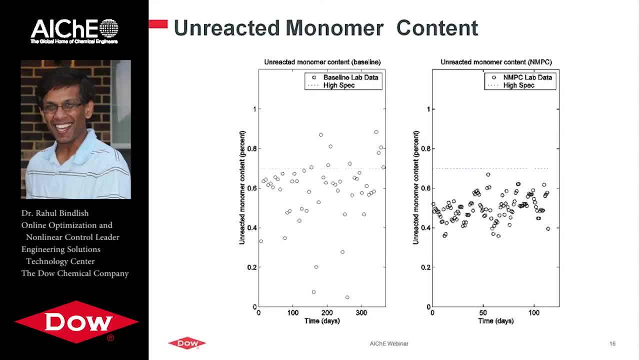 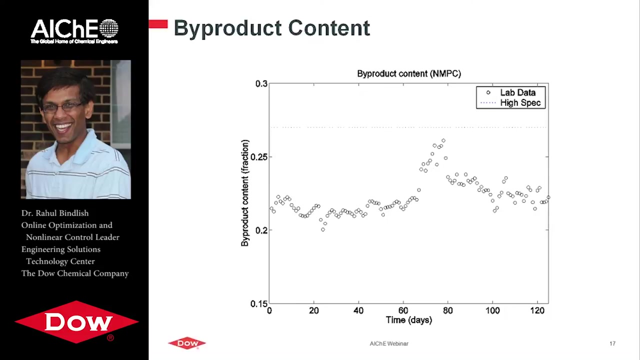 we've been able to run this controller and the process without excursions on unreacted monomer content, so we've been able to keep it within specs. So the other thing to notice after the controller ran for about a year or so. 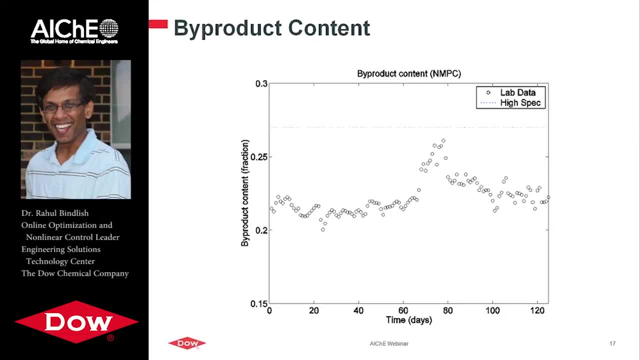 then we ended up deciding that we would like to add another control variable, which is the byproduct content. It's an economic measure of the process, so we didn't even have a lab measure for it, We just had a simulation result for it. 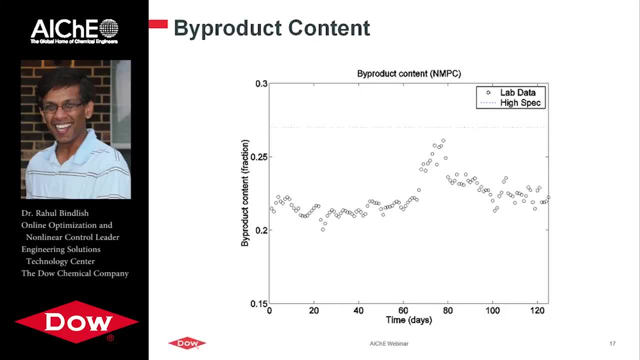 So the old controller couldn't do anything. I mean, the old simulation model just had a simulation of that, But we didn't have a lab measure for it, so we were sort of trying to minimize it but running it without any lab measure. 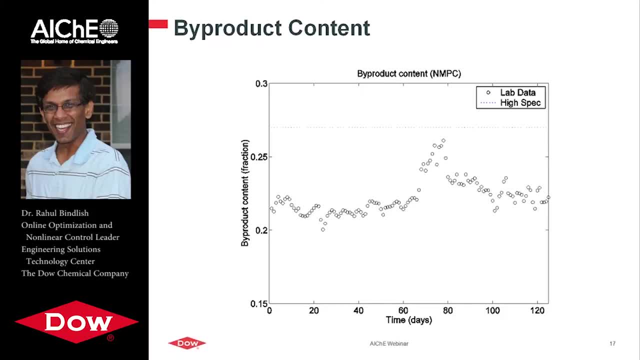 But in the new controller we added the lab measure for it, added the models for it and we've been able to minimize the byproduct content when we can. So this graphic shows the spec of that byproduct content, which is like .27 or so. 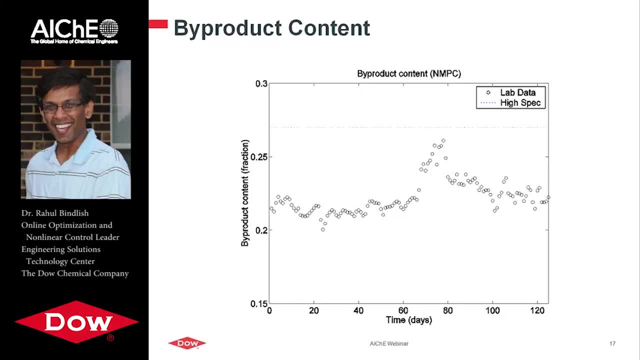 So we've been able to keep it much lower than that. But when needed we have to let it rise as needed. So in this case it actually has an excursion all the way to .26, but it still stays below the spec limit when needed. 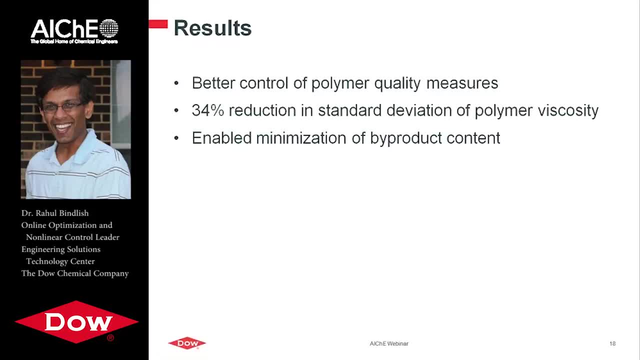 The results. we have better control of polymer quality measures. We've been able to do that especially for polymer viscosity, unreacted monomer content, and we have also added another controller objective that allows us to minimize byproduct content. Now talking about reduction and variation in polymer viscosity, 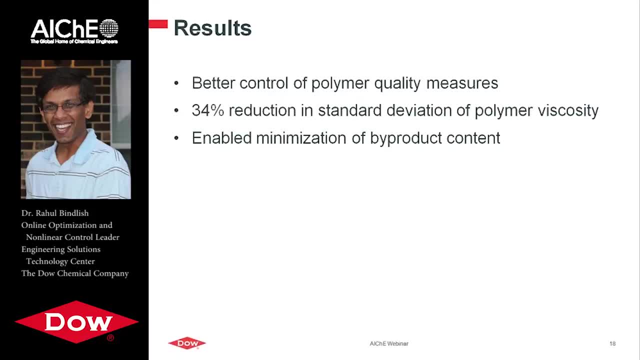 because that was the original charter of the project. we've been able to reduce the standard deviation in polymer viscosity by 34%, And we first chartered the project thinking that we should be able to do about 20, 25%. So we've been able to do slightly better than that. 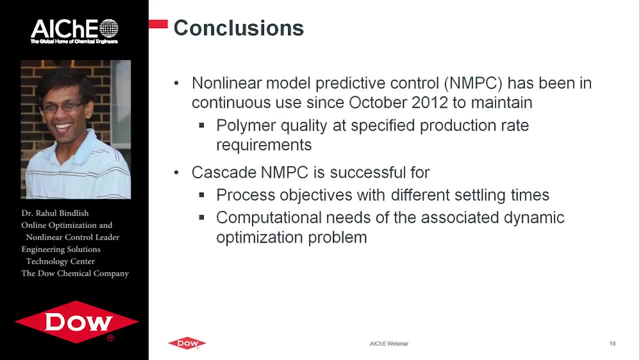 This controller has been in continuous use since October 2012 to maintain polymer quality at specified production rate requirements. so the production rate requirements are changing depending on what's happening in an upstream plant. So we undergo a lot of feed rate disturbances and such, and we have 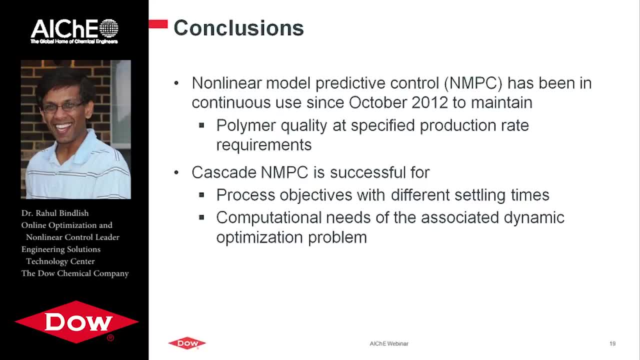 to maintain polymer quality while those rate changes happen. The cascade nonlinear model predictive controller structure is successful in an industrial setting. It allows us to achieve the process objectives that may have different settling times and may even have linear versus nonlinear. It also allows us to address the computational needs of the associated dynamic optimization problem. 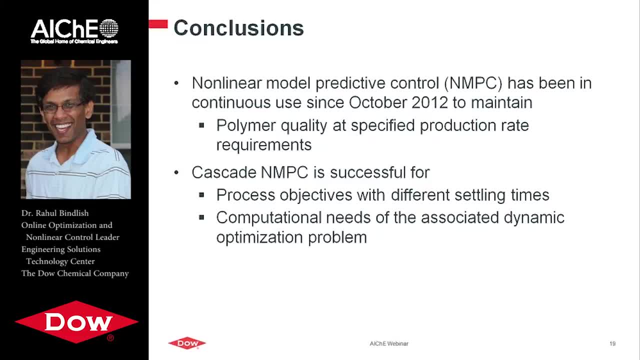 so that we can run the controller in real time. I'll mention one more thing. After the initial success of this project, what has also happened is we have now two or three more active projects that we have been working on, based on the initial success of this project. 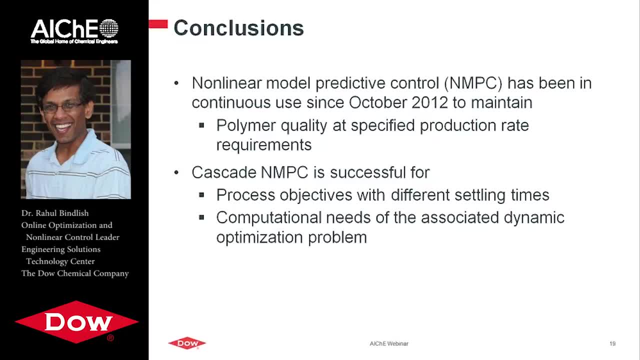 So it's been a long journey. Apart from the technical learnings on the technology and process that I shared with you today, I also want to mention, as we do these things, one of the things, especially in an industrial setting, as we increase or enlarge the scope of the controller to make it successful. 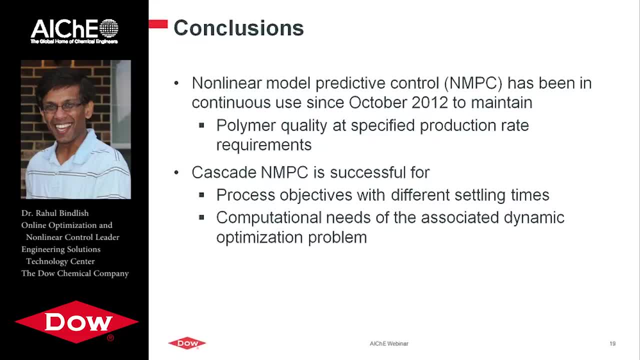 to address the plant problems is to have the partnership with the plant people and learn from them as we implement these solutions. That's all I have to say today. At this point, I'll be more than willing to end the session. I will be happy to answer any questions or comments that you may have. 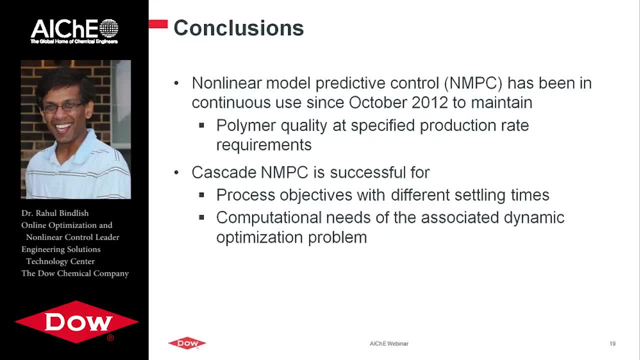 Okay, fantastic. Thank you, Raul. That was an excellent presentation. We'll go ahead and open it up to questions now. If you'd like to either unmute your microphone, you can ask a question, or you can put a question into the chat window. 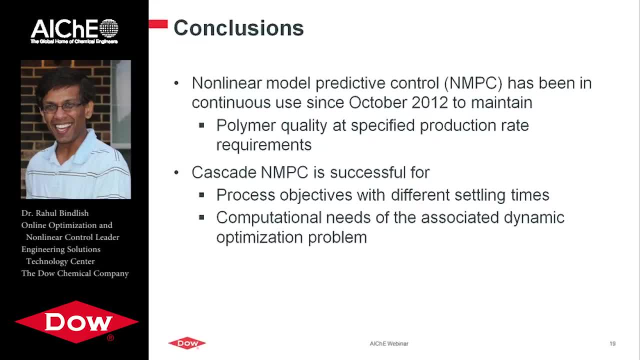 And so, just to start, we have one question from Mike Tay. He asks: Was the fundamental monitor common? And then, if steady state, how were the dynamic models in the NMPC developed? Okay, well, the fundamental model. we had both the steady state, representation of the fundamental model. 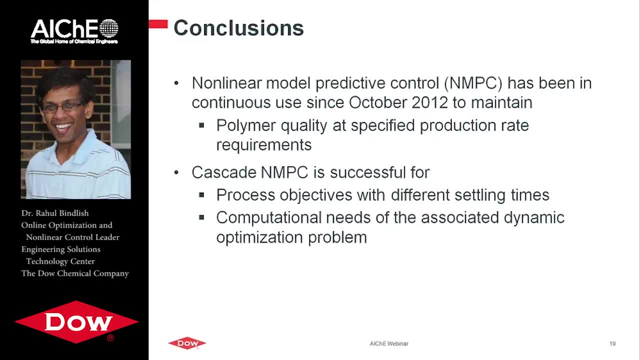 but it essentially was a dynamic model and we have the dynamic model. We had the fundamental dynamic model and we used that to establish the dynamics. But in addition to that I want to mention we used the model to come up with our initial models. 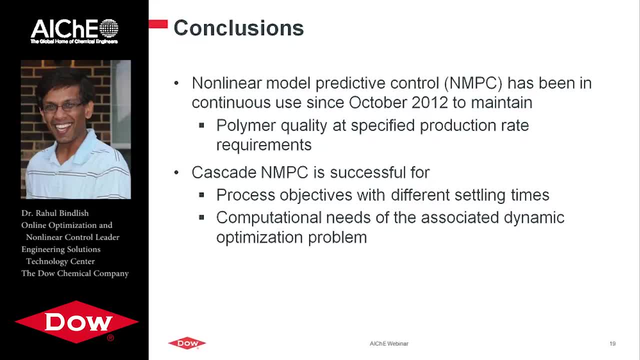 So we fine-tuned our models because a plant does not. I mean, our models are an approximation of the reality. So, even though we had a dynamic model, we had to fine-tune some of the observed dynamics slightly for some of the control variables, based on what we saw in the plant. 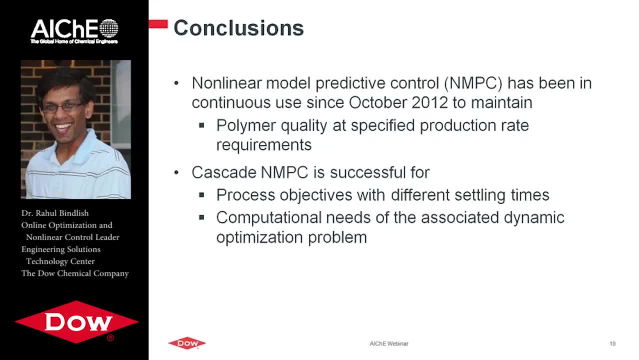 Okay, Thank you, Thank you, Okay, fantastic. We have another question here: Bounded derivative networks, the models that are used supposedly in that outer loop. have you had to go to any new grades, new products that you're manufacturing? 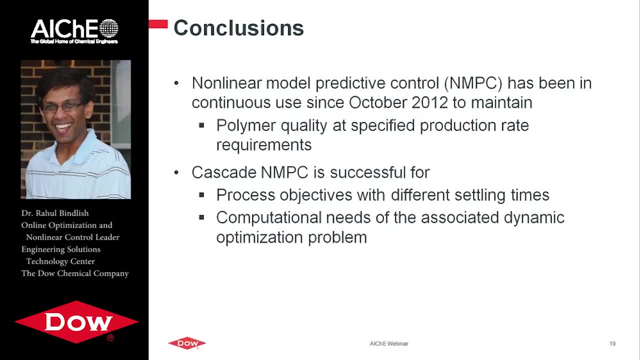 and how do the models extrapolate? You know what's the process of maintaining those models? Excellent question. So that's been great, That's been. I think that's really one of the most interesting challenges, as we have learned the process and also gone through those learnings. 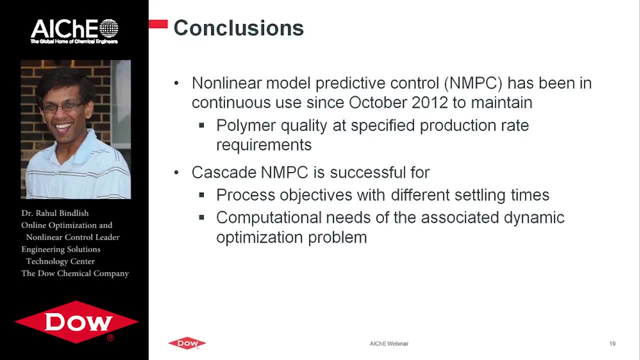 So one of the things that happened is when we went to lower rates, we had to develop new models and we saw learnings. So the models extrapolate reasonably well, but there's some tools in the software itself so we have to ensure monotonicity to make sure they extrapolate well and they are relevant. 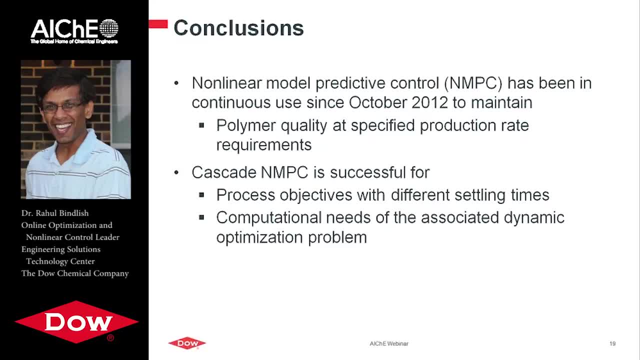 So we don't have. so we have to examine the models and we had to do a lot of model work to make sure the models were not overparameterized and did not have higher orders unnecessarily, and that would result in poor extrapolation. 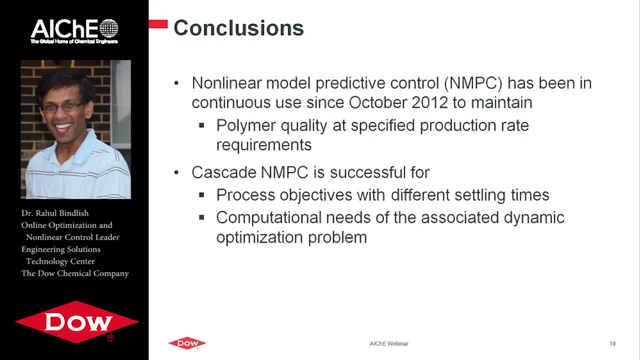 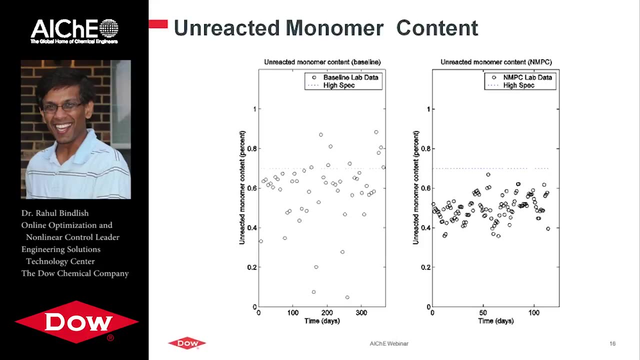 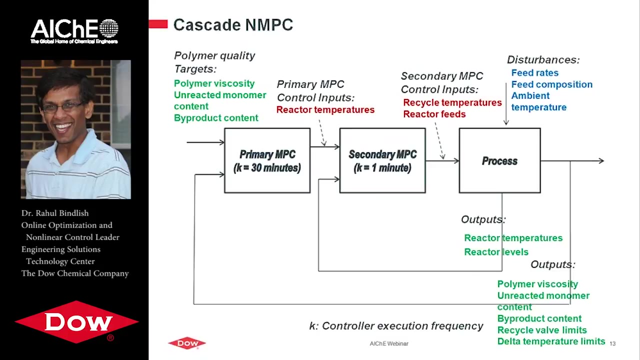 So we had to examine the models and the first derivatives very closely. Okay, great. So we have another question, And maybe you could go back to the slide where you show the primary and the secondary MPC controllers. But the question is, why does the process need to have a secondary MPC controller? 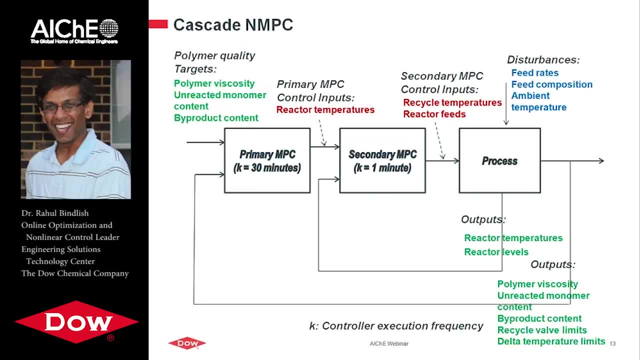 Good question. So in the past we were controlling the reactor temperatures and levels using a DCS control, But by having an MPC controller for that, we were able to control the reactor temperatures and levels a little better than a DCS strategy, and we were able to use recycled temperatures and all the intermediate reactor feeds. 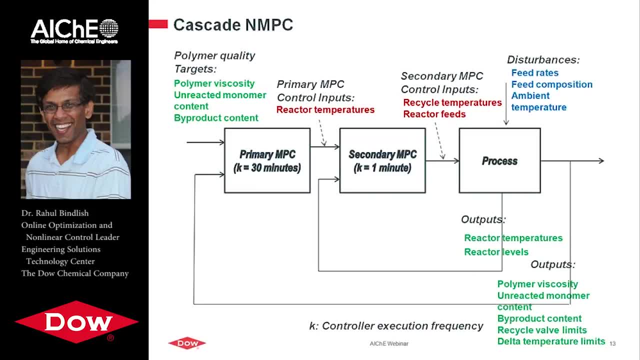 to maintain all the reactor temperatures and levels simultaneously, and basically it's a better setting. That's all. We were able to take advantage of the multivariable interactions instead of single input, single output pairing in a DCS. Great, Okay, we just have another question here that just came in. 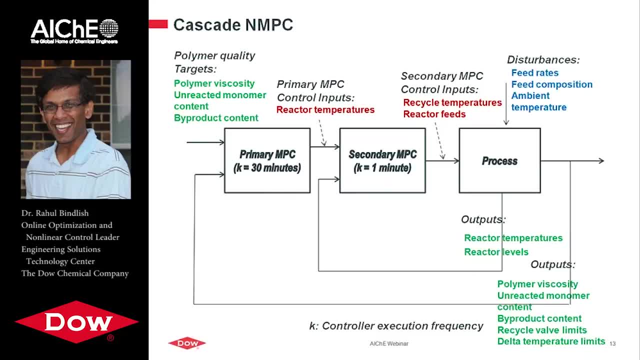 What processes are included in the model other than kinetics and heat transfer? Are the kinetic parameters estimated? So in this case we had the nice thing: the business and the technology people had already been using this model to develop their process and had validated this model. 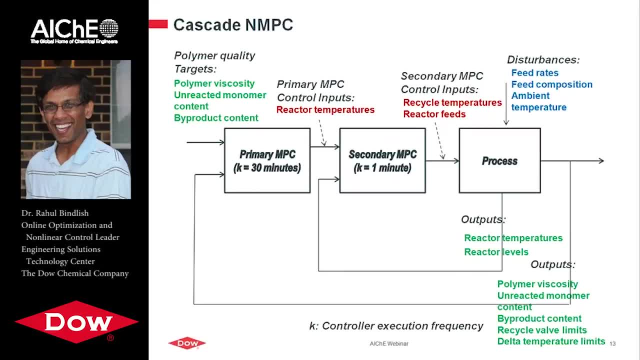 So they had the validated static parameters. We didn't have to do estimation of the kinetic parameters, so they had validated this model with planned data. So we had a validated model, so we didn't have a need to do that. Okay, great. 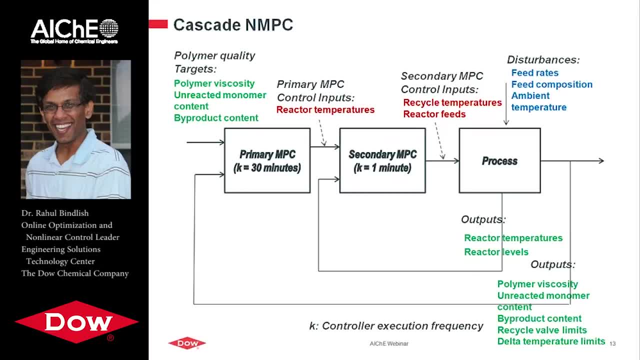 And then I guess the other part of the question is what processes were included in the model. So was it mostly the reactors or did you have some of the finishing areas? What was the scope of the model? The scope of the model, essentially, was the reactor area, not the finishing area. 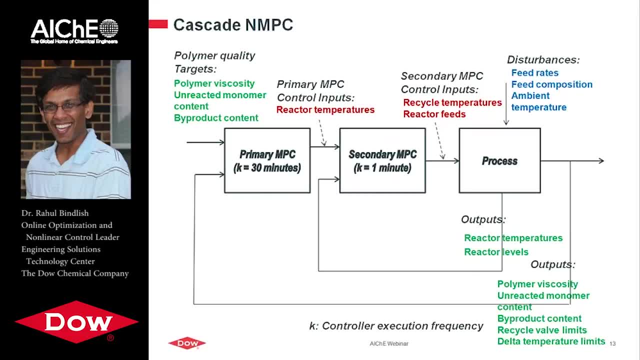 The finishing area we approximated by simpler things. so the scope of the kinetic model is the seven reactors in series, and that's really the big part of the model anyway. Okay, great, Okay, let me scroll down here. Okay, where are the NMPC models in the cascade framework? 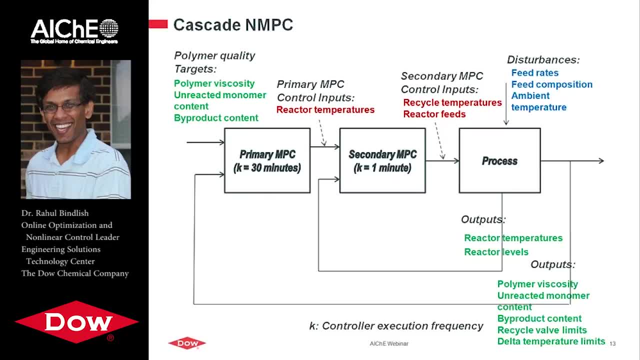 implemented Software. How are they solved via solvers? So just a question about where are the NMPC models in the cascade framework implemented, and then how are they solved with the solvers? Okay, very good question. So this actually reminds me of my graduate school days somewhat. 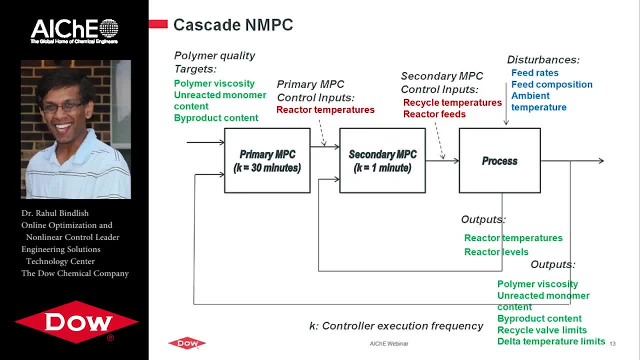 So when I had the freedom there, I could write code wherever I wanted to write and I could use some of the NAG routines and some of the state-of-the-art optimization software In an industrial setting. I don't have that luxury. 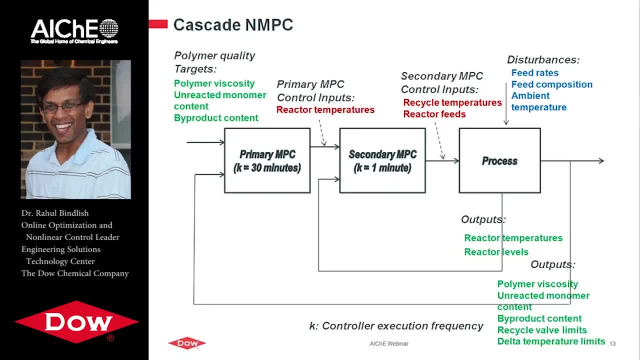 So the NMPC models are in the primary model predictive controller and they're implemented in the Aspen nonlinear control framework, which is a BDN. They're implemented as BDN models and they're implemented on a server which is at the plant. 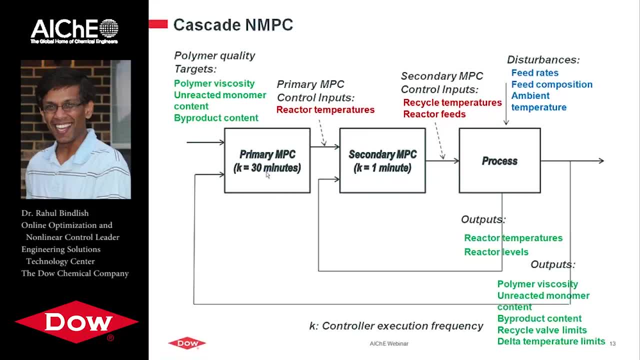 And we basically have to use the optimization algorithms within that controller. So we have to make it work to come up with the right answer. so we do that and make sure it works in that framework. Okay, great. Another question: How well is the estimator working in identifying the states from the outputs? 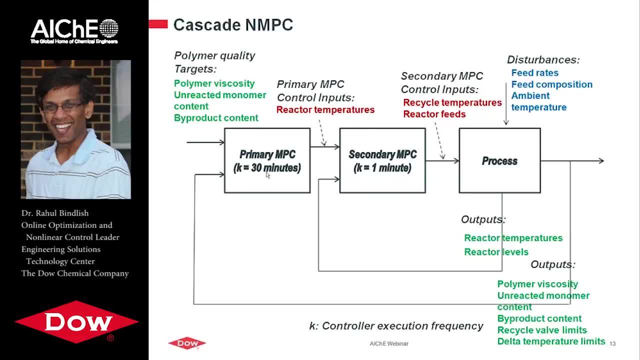 Any negative concentration estimates? No, we didn't see that. We didn't see the negative concentration estimates, So we haven't seen that as being a problem for the problem we are looking at. That's something to watch for, especially with an extended common filter, absolutely. 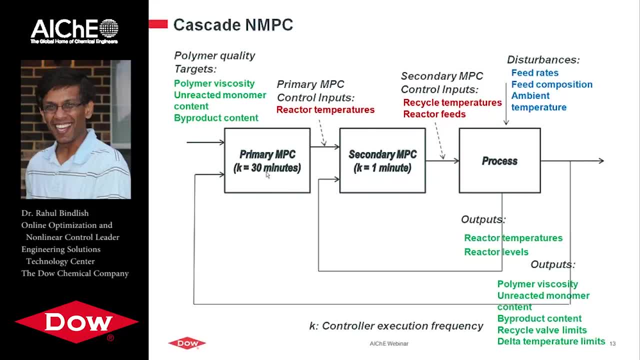 Was it very hard to tune the filter? It was hard, but not as hard as I would have thought initially. to be honest, I think if we had the right noise dynamics or the variance initially, we actually were able to do what we needed to do. 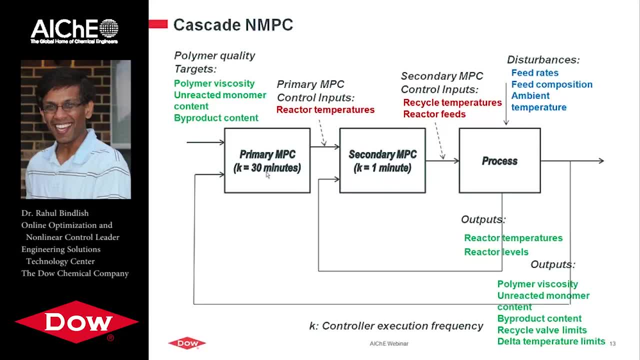 without having trouble there. Okay, so another question, A question on batch processes versus continuous processes. So the question is: are the processes shown in the slides continuous? What is your idea on application of your method to CSTR or batch processes? Okay, the processes shown in these slides are continuous. 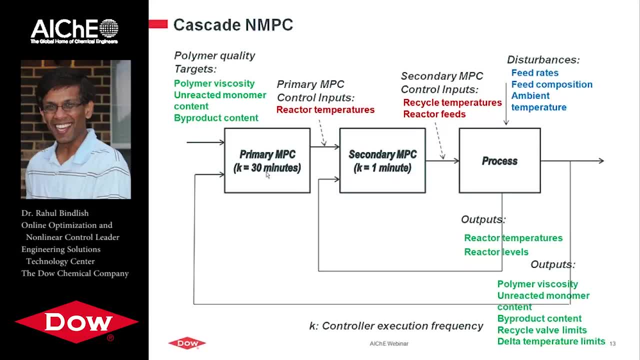 So going to the CSTR? yes, the controller and the map here applies directly. In a batch process the objective is different. The objective is not to minimize batch time and we're not going to get as much continual disturbances, so we don't have these disturbances that are hitting us. 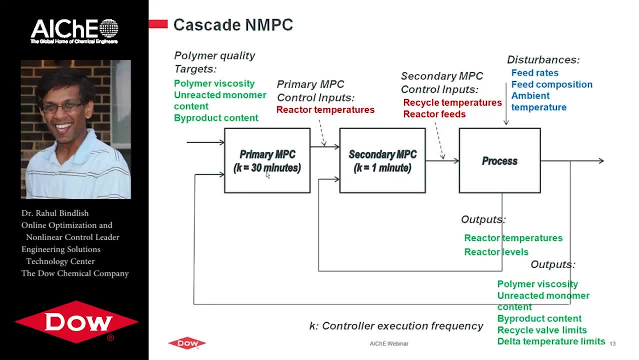 But we have lesser disturbances that hit us and we are able to control the batch better. but we have to minimize the batch time. So it's a different controller objective and we are looking at and that's something that would be a different controller objective. 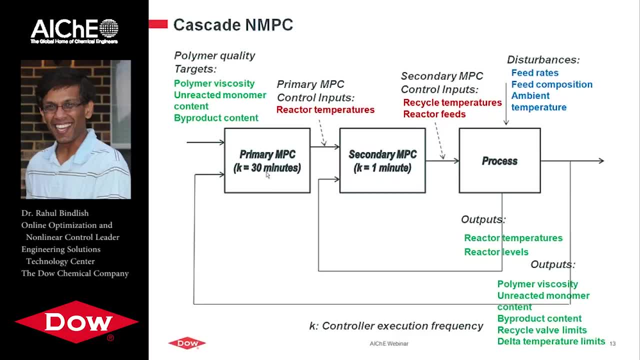 It won't be this controller formulation, Great, Okay, so we have two questions that are very related. I'm going to go ahead and ask the first question first and then we'll get to the second one. Is the process model used in the primary NMPC retuned in another loop? 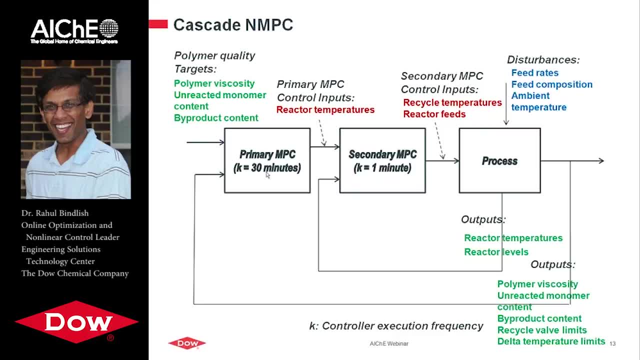 offline, manually, or is it rarely retuned? So what has happened is: we have been asked to, so we have added or examined the models or extended the models to different operating conditions. So, in this case, after running the controller for a year or so, 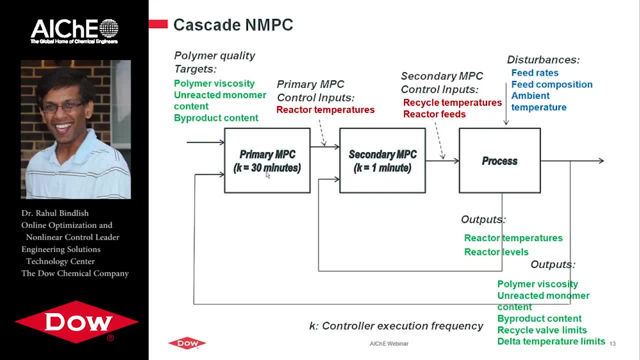 we ended up developing the process. We ended up developing models for lower feed rates- 35 percent versus 60 to 70 percent. We also came up with models that would work with six reactors instead of seven reactors. So that's one thing that happened. 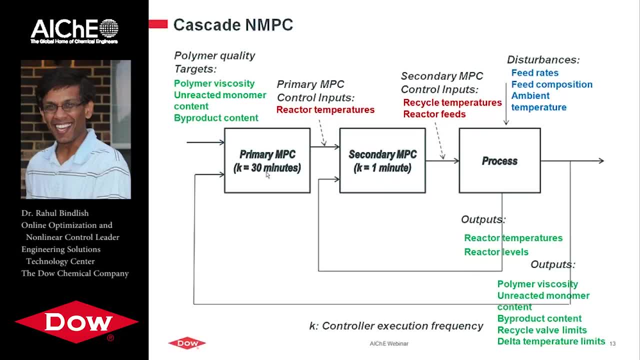 So, as far as retuning is concerned, I think there was a lot of retuning of the models when the initial deployment happened, So there was a lot of that, But once we did due diligence and we did our hard work, it was less of a requirement. 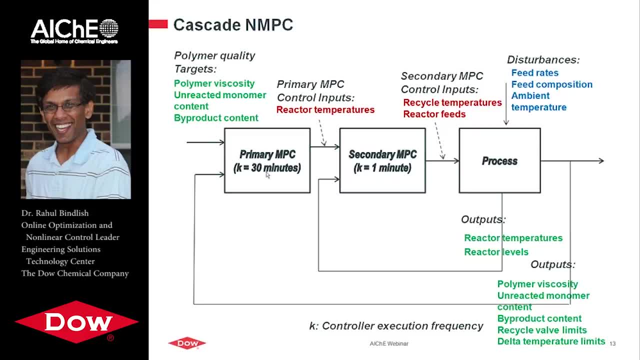 What happened after that was more of the requirements had changed. They wanted to run at lower rates, They wanted to run at six reactors or seven reactors. So I think the requirements are always going to change in an industrial setting And when you first deploy the controller, 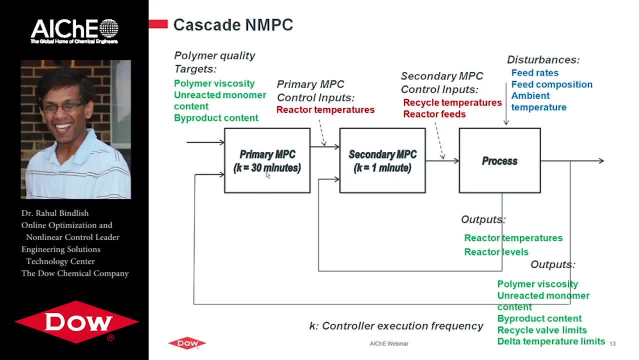 even if you have done everything you have done, there will be a lot of examination and tuning for an extended period of time to make sure everything works properly. And in this case we want to do that, because what happens now is based on what happened. 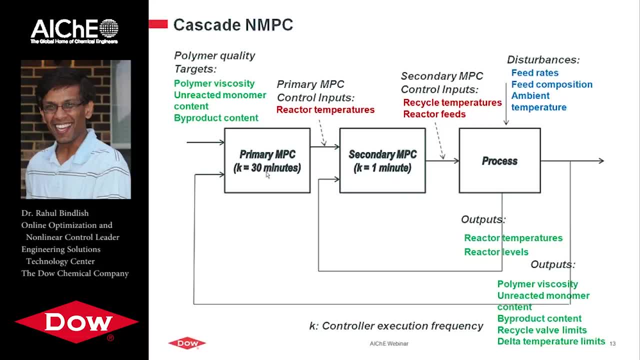 seven or ten days earlier. So the nice or bad thing is, if something is good now, you don't see the effect of it until seven or ten days, and then it's too late. So you just want to make sure you have what you need. 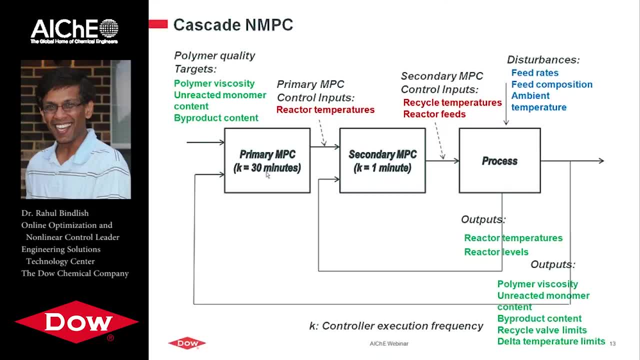 and you have to answer those queries and collaborate with the plant and technical people appropriately. Okay, great. So the follow-up question. the second one: can you just give us some insight as the process is changing? how is the nonlinear model updated? 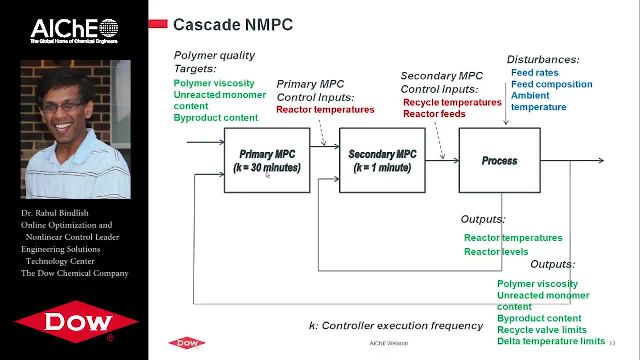 Do you have to start from scratch, or can you start from the prior one and then update incrementally In some cases? in most cases, we can start from our existing knowledge, But I think the bigger thing to me is it's not a turnkey project. 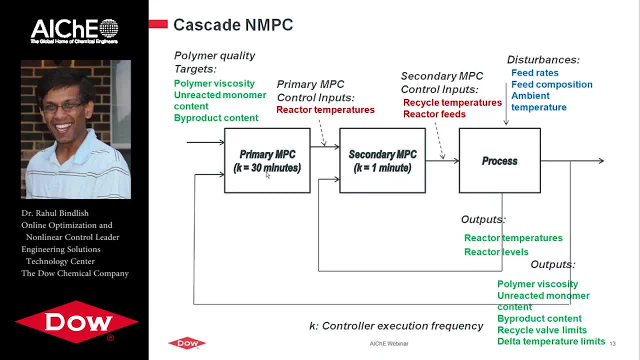 the way we do things here. So we have the – I have made sure I have the appropriate engagement with the appropriate people at the plant and tech center level, So even have – when we first deployed the controller, we even had a weekly placeholder meeting for like months or about a year or so. 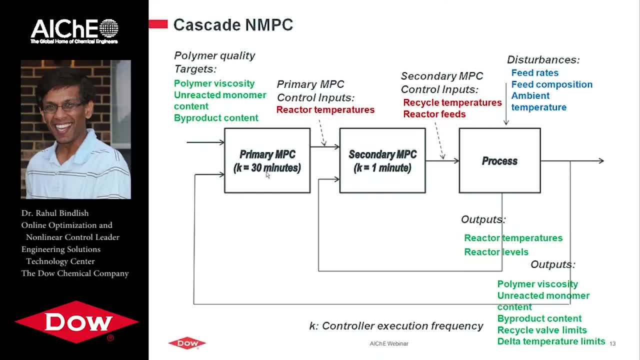 So it allows me to watch this controller. This was the first one that we had done at Dow and we wanted to make sure it was a success. Otherwise it would have been turned off and said, okay, this was doing crazy things. 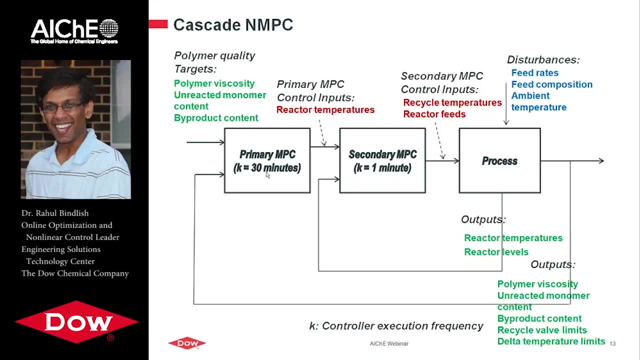 These guys came and tried to do something. Let's turn it off and end the story. But because we engaged them and learned from them and also made sure they understood what the controller was doing or why it needed to be retuned, then only they would allow it to run. 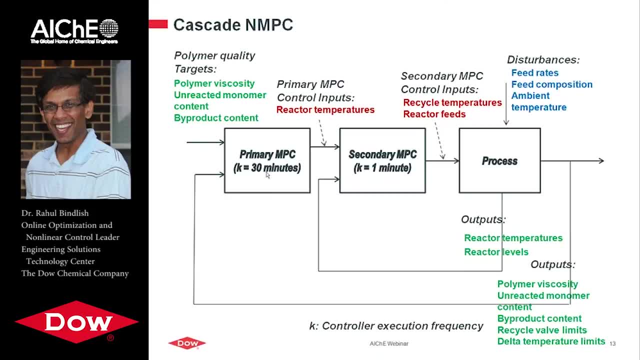 especially on Friday night and Saturday night when they are in the control room and they are managing the emergency, not anybody else. So that's the insight. I think in my mind that tuning can happen as a small tuning, but there's a lot of process knowledge that needs to be assimilated. 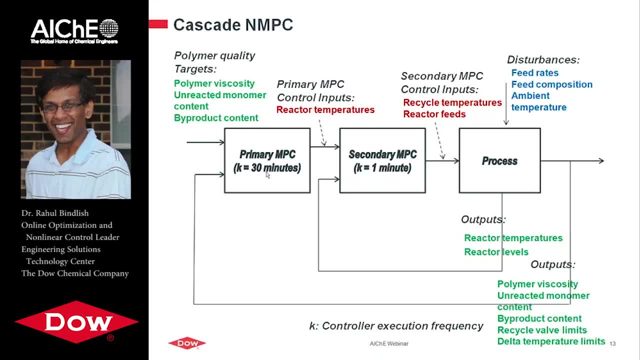 We never had to rebuild that controller from scratch, But it was more a question of understanding what the needs are and basically doing the right thing for the process. Great, Could you go to the slide where you showed the before and after with the product quality limits? 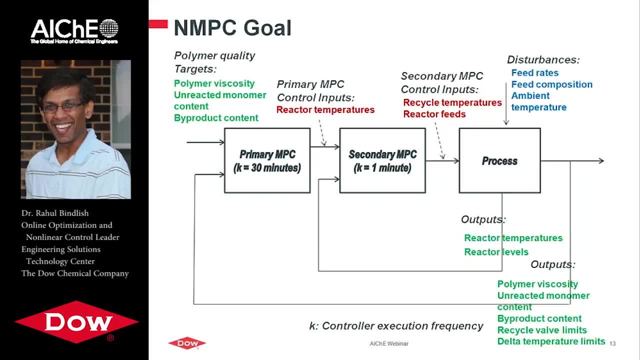 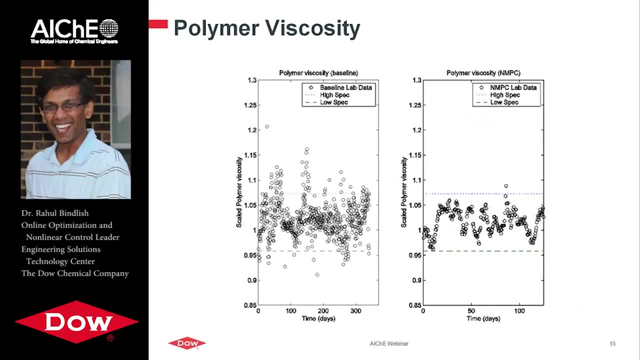 With the what. The distribution that showed the Okay. so the question related to this is: is there a limit or band for the control outputs before the NMPC performs a control action? So let me make sure I understand that question. So the limit for what? now? 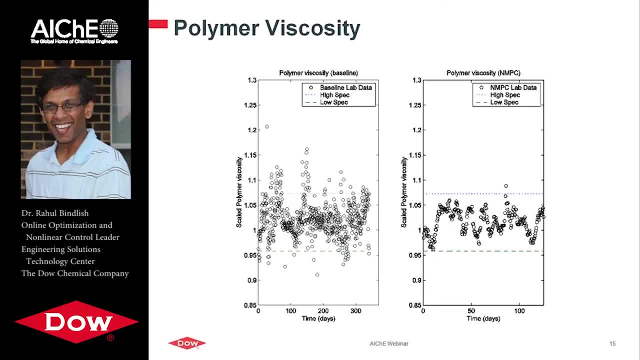 So just the question is: does the controller only ask when it predicts it's going to be going outside of this dead band, or is it always trying to drive to the outside? Okay, good question. I guess this doesn't really show it very clearly. 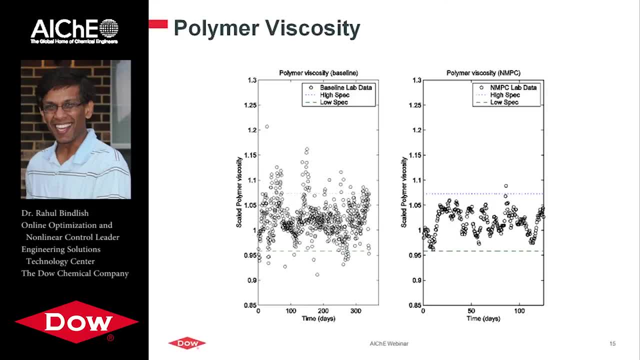 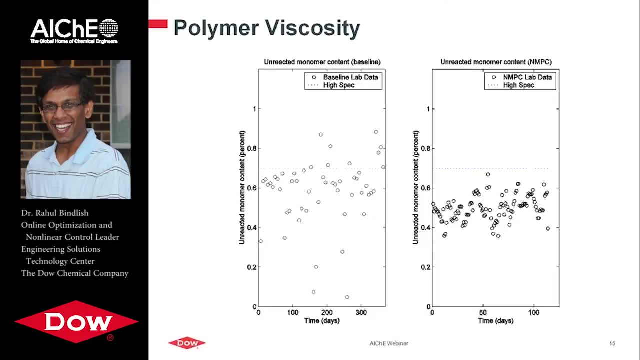 So the polymer viscosity, we are controlling it to our target. So that's the only polymer quality attribute we're controlling to our target. The unreacted monomer content: we are not controlling it to our target, We are just trying to make sure it does not have an excursion. 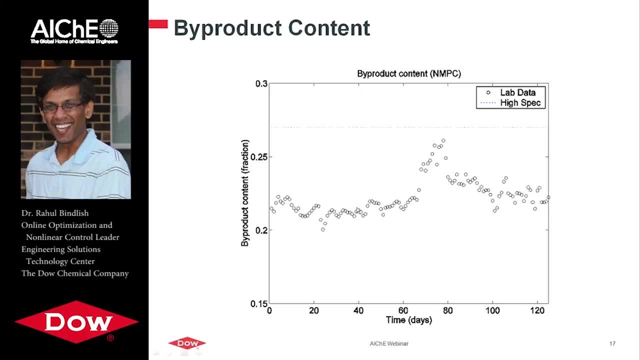 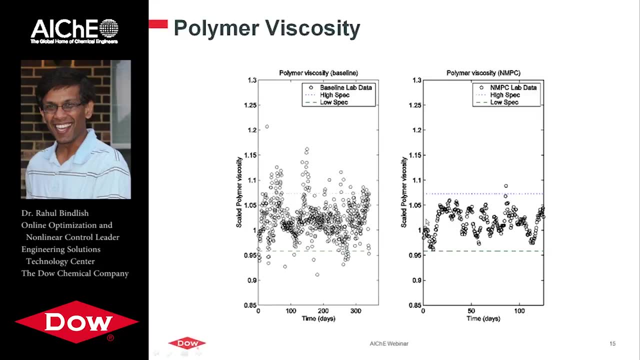 And the byproduct content. we are always trying to minimize it. So this one- the first one, the polymer viscosity- we are controlling to our target. I didn't show it here and it's really in the middle here. We're controlling it to our target, but we also have the spec limits. 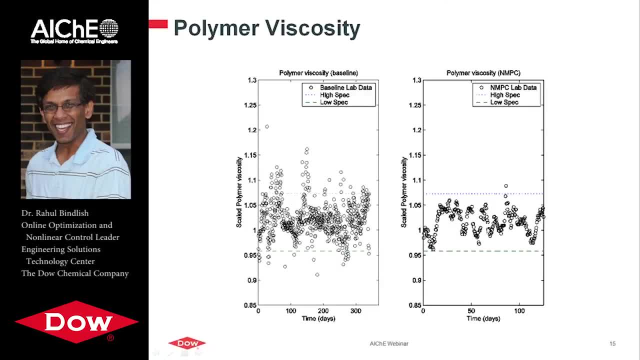 that are very important. So there is a value in controlling it to our target. So we are controlling it to our target, Great, Okay. so we have a question, And this individual had a question about your first principles models. You said that you at Dow, had these validated models. 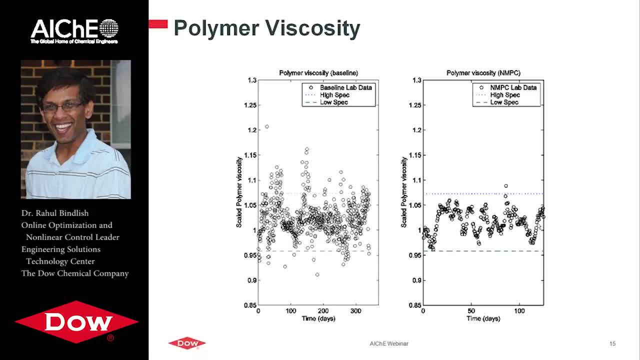 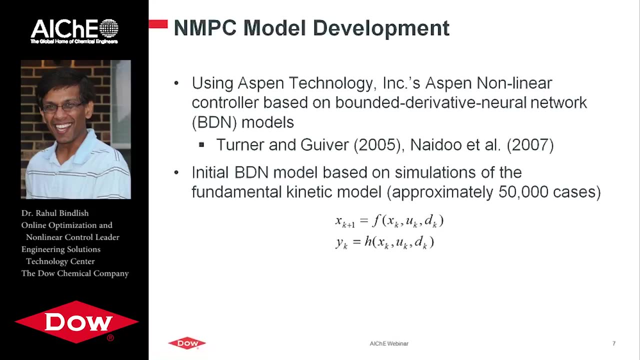 And then the question is what would be an advantage of using a first principles model versus a states-based model or these empirical models, and any challenges that would arise in splitting the controller into two, with the first principles and possibly linear model or empirical model? 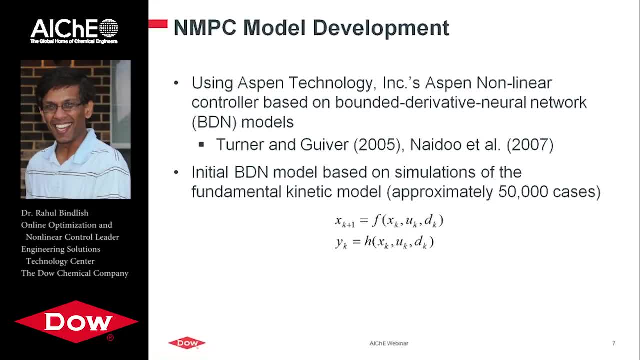 Okay, I'll try to answer. I think I understand what this individual is getting at. So in my mind there's some things here. So we have the first principles model and for some of the finishing and mixing kind of areas we may have some empirical representation. 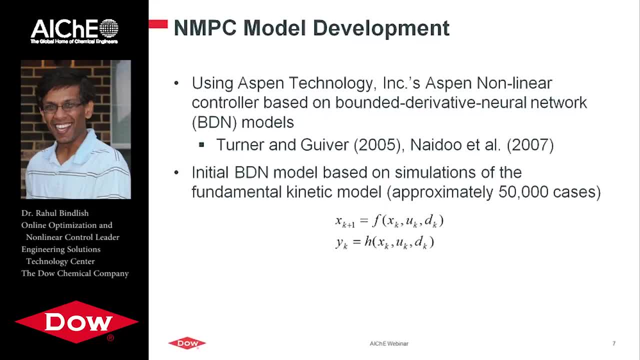 And those are adequate and have the appropriate physical insight, And we use that and that's what we call our fundamental model. So it's the first principles, with kinetics and also some empirical representation that captures the mixing and the finishing area. So that's what we have. 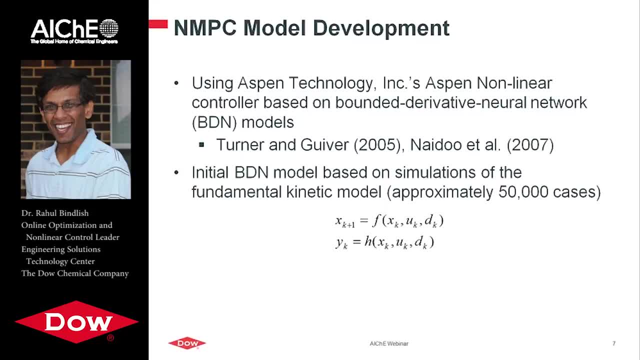 Now the question is the advantage or challenges of doing that compared to using a BDN model. We needed to use a BDN framework because we wanted a commercial control solution in the plant that's sustainable, So the challenge here was to ensure that the BDN extrapolated well. 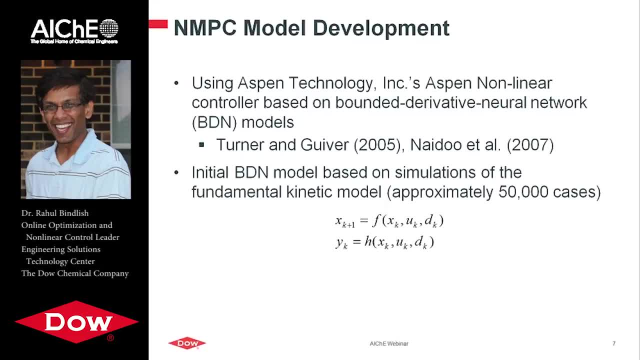 without creating instability. So that was a challenge. We examined the model prediction, the first derivatives, all the manipulated variables, against the polymer quality attributes and examined them for monotonicity and made sure they made sense. So we had to do that, Otherwise we would have problems. 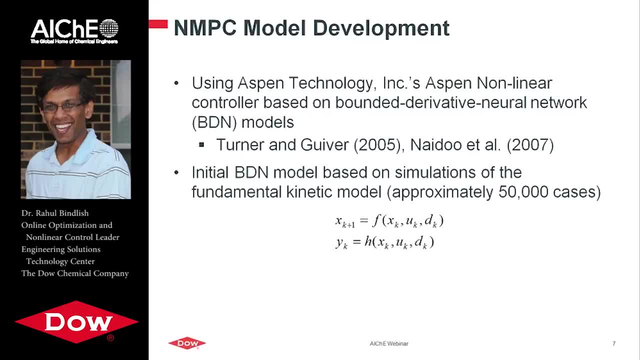 And with the first principles model we wouldn't have to do that, But we didn't have the luxury of using the first principles model correctly. Great, Okay. Well, I think we're about out of time. now. We have more questions than we have time to answer today.